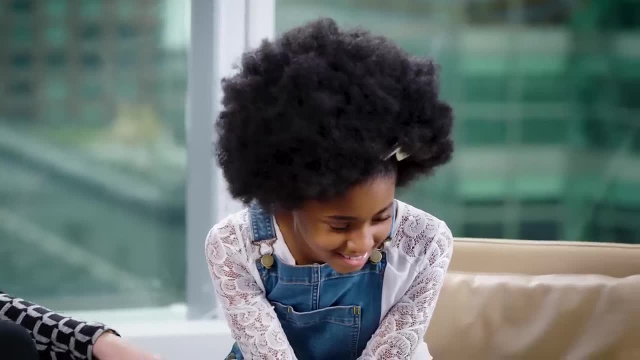 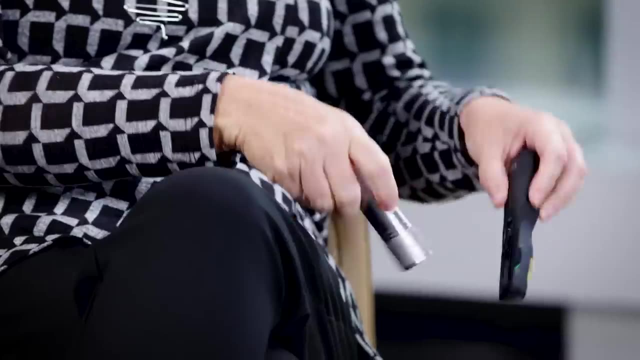 Yeah, And one of the fun things people do with lasers: the cat will try to grab that dot. I'm sure what you have at home is a flashlight. I brought a cute little one. So the question is: do you see any difference between what a flashlight does and what a laser does? A flashlight 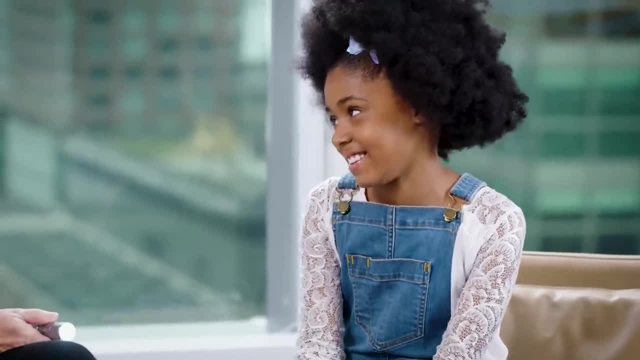 is a bigger um sign and the laser is just a dot. That's true, the laser's just a dot, And so the other thing to notice, though, is that this seems like like, when I think about it, I think about the laser as a dot. I think about the laser as a dot. I think about 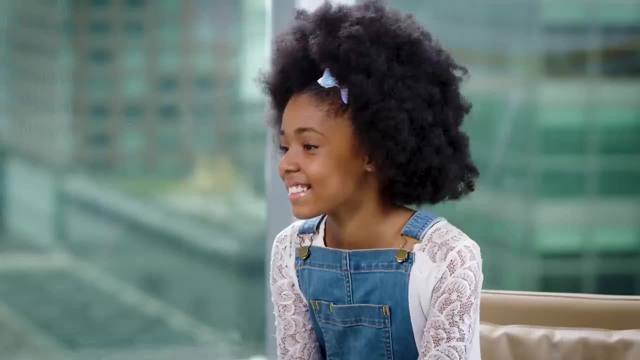 the laser as a dot And I shine it in your eyes and I'm sorry if I do, but it seems awfully bright, doesn't it? And yet, when you know, you shine this down and you put the laser- which one do you see? 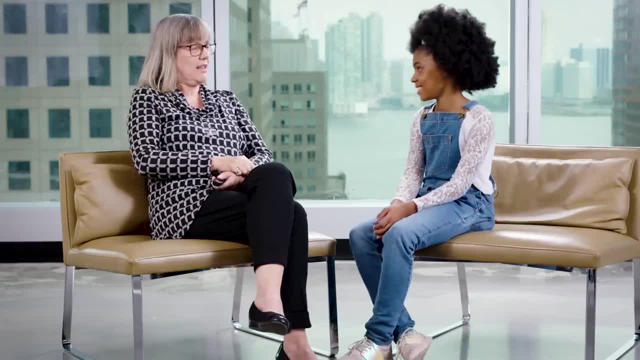 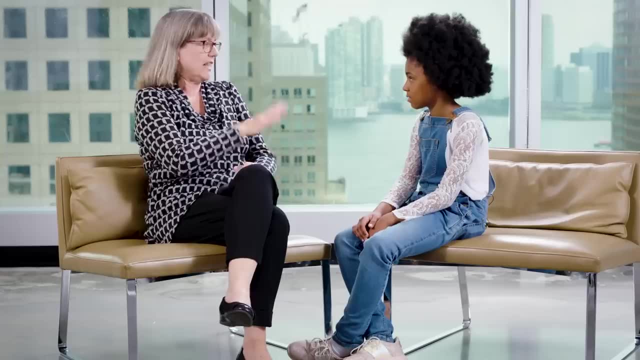 easier? The laser, The laser? So which one do you think's more powerful? The laser, And yet it's not. Isn't that amazing? Yeah, One of the things that lasers are great for is that because if it's a directed beam, we can actually put that light. 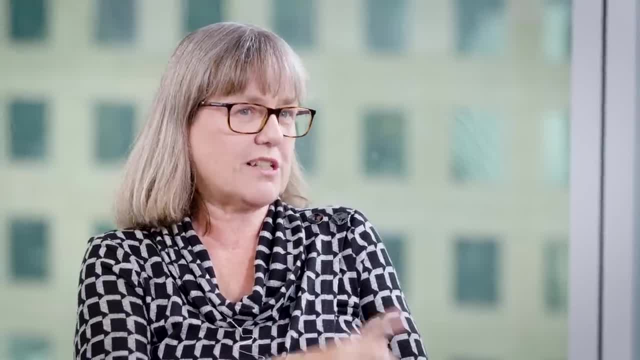 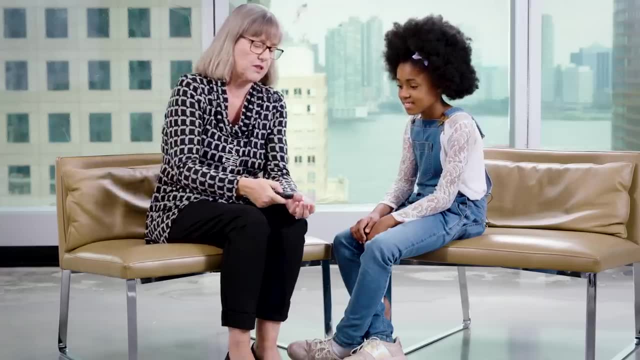 where we want the light to go. And sometimes we maybe just want to see something around a corner and you can't see it. But with a laser you can actually- and this is a smoky one, so you can actually watch it go. You see it actually bending the corner And that's because the light 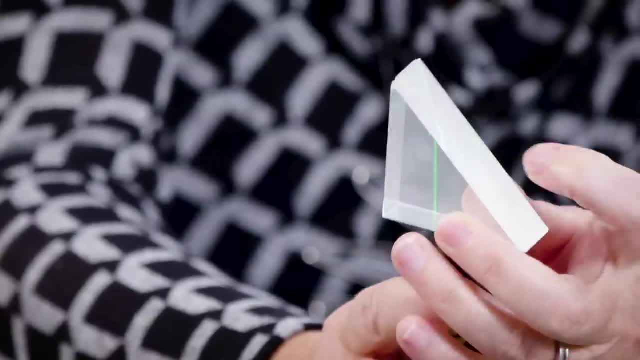 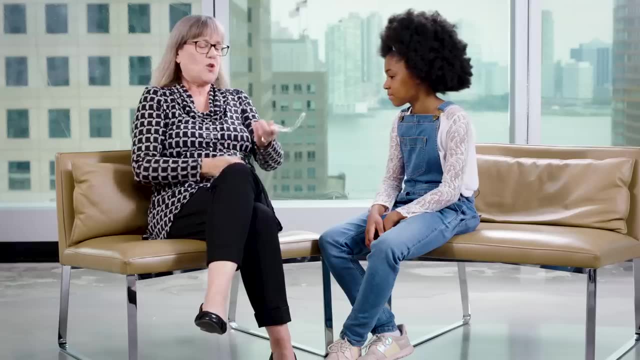 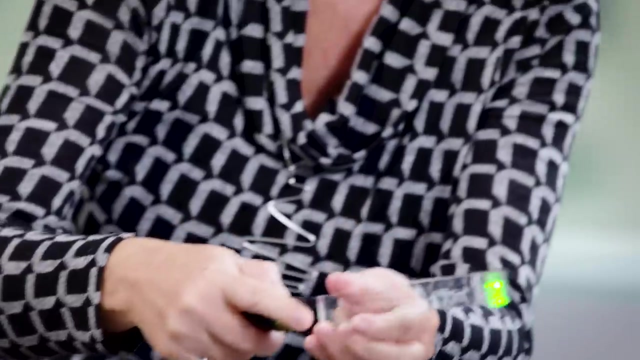 will go through this glass, but when it hits that corner, it has to bend And we actually send laser beams down. glass fibers the size of your hair. Yeah, So this obviously is much bigger than our hair, right? Yes, So this is just a demonstration. If you have a laser like this, it actually 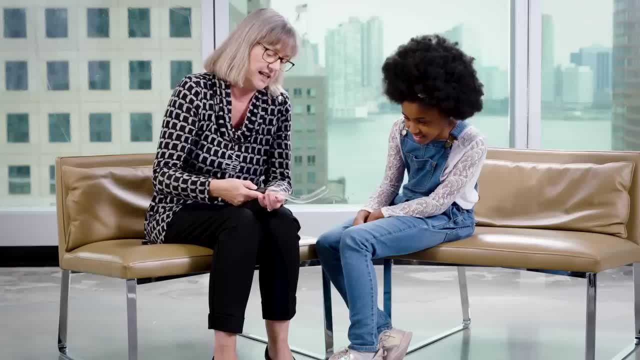 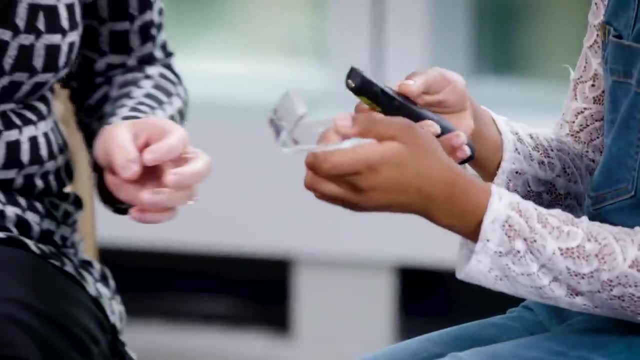 bends and comes out. I'm going to point it to you and you'll see it coming out the other end. It hits these walls. It has to go around and come out the other side. Do you want to play? So, is this the first time you've seen a laser, or have you gotten to play with lasers somewhere else? 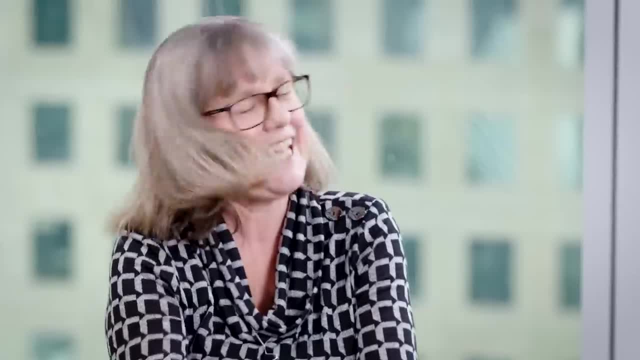 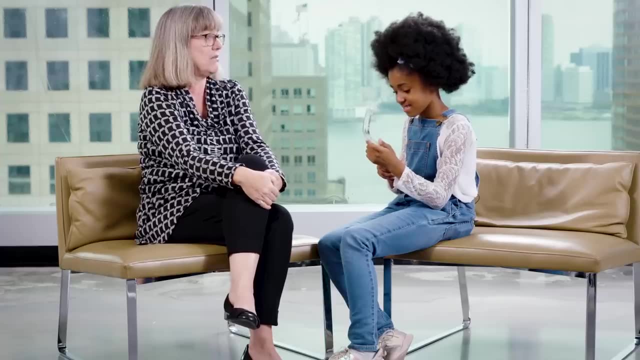 I don't have a cat toy, So you don't need a cat toy. no, Have you ever gone to a grocery store and just scanned your objects over? Yes, Have you ever seen that? maybe there's a little bit of a red light when you do that? Yes, That's a laser. We cut steel with them. now We actually do surgery. 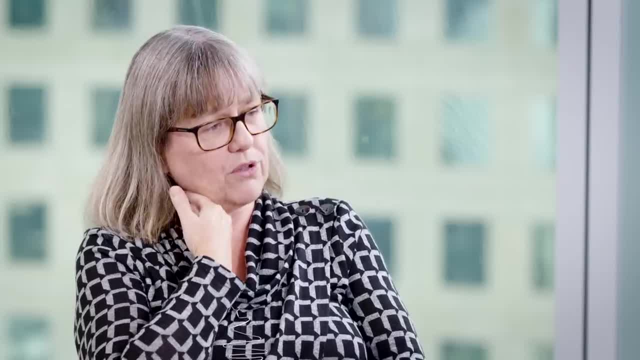 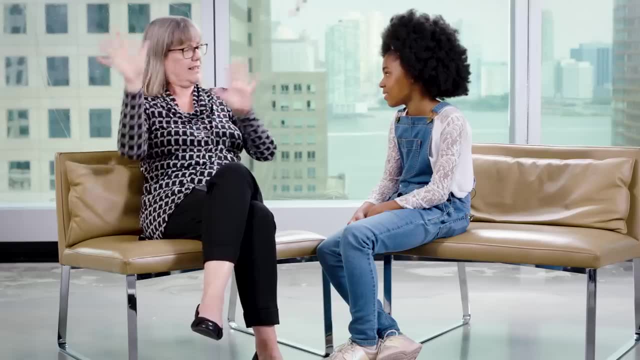 With lasers. you know, when some people have either scars or birthmarks that they don't want to see, we can actually remove those with lasers. now We've never seen a laser light show. When they light up the sky with lasers, it's almost like fireworks. Wow, I saw a shooting star. 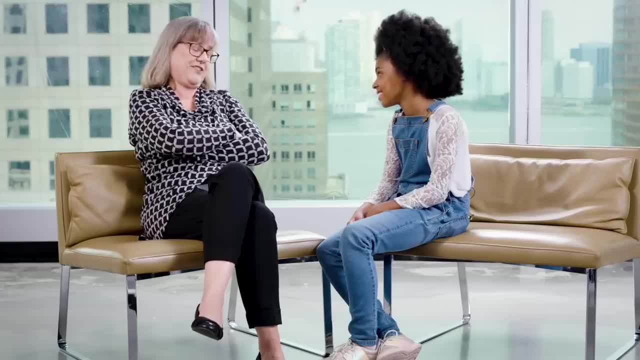 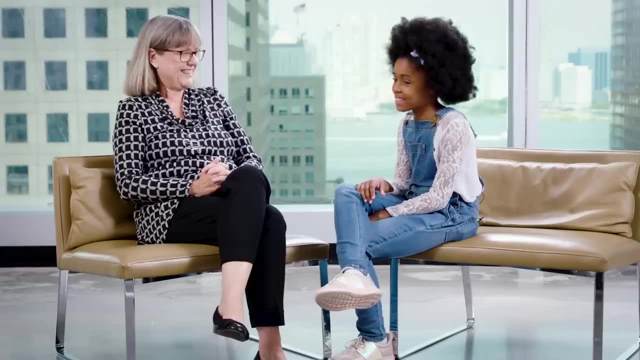 Oh, you got to say a shooting star. Well, that's, that's cool. That's nature giving you the show there. So what do you think about lasers? You think they're fun? Yes, they're very cool, And I like the green, the one with the green one, The green one. And the next time you go to a 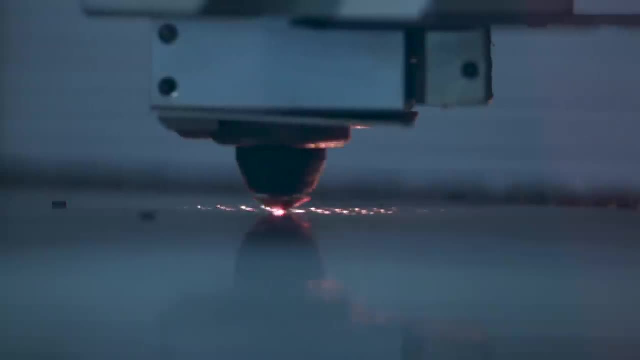 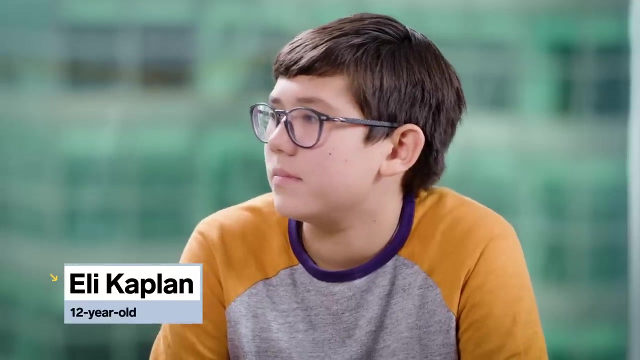 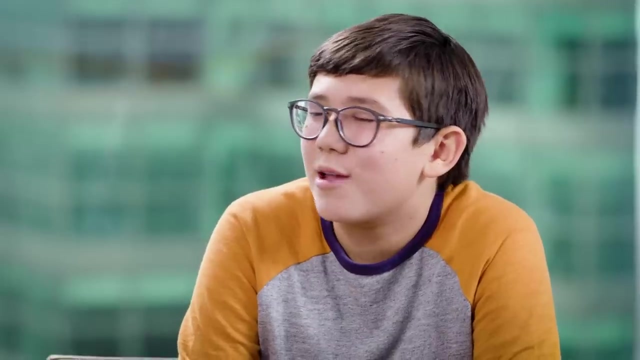 laser. take a peek at the red. Okay, Today we're here to talk about lasers. So what do you think about lasers? I think they're pretty cool. They show up in a lot of my favorite books and movies, like Star Wars or just a bunch of. 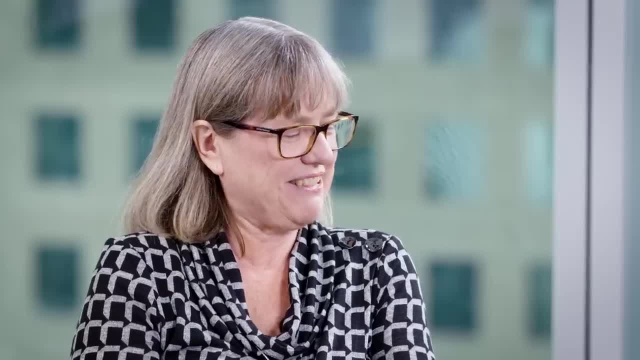 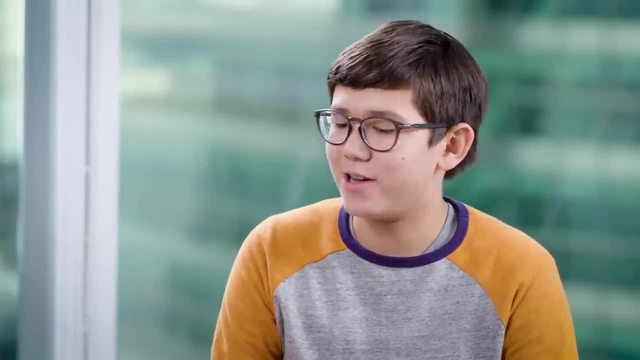 different sci-fi movies and books? Do you know anything about lasers? What makes a laser special kind of light? All I really know is from like sci-fi books and movies and like the factory cutting lasers that they used to like cut steel and stuff. Do you even know, maybe, how to make a 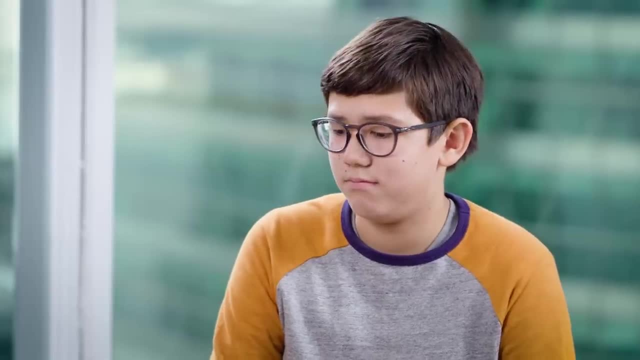 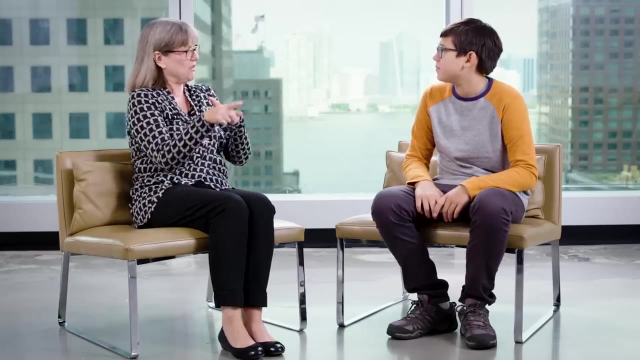 laser that it would be strong enough to cut steel. No, Oh, okay. So one of the things about lasers is, if you've ever seen a laser beam, you know it's very directed. Like: what are they made out of? What is a laser made out of? Well, really, it's sort of the same thing as a light bulb, right? 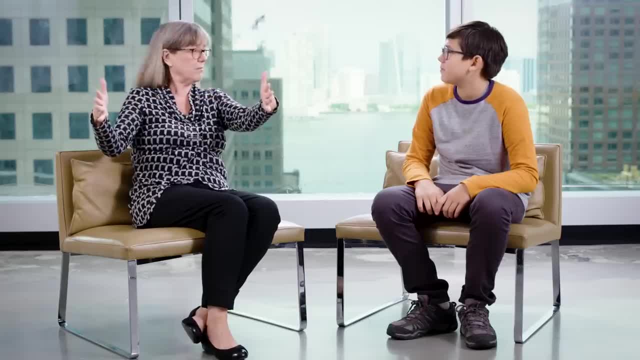 Because people- So it's a beam, So yeah, it's a light bulb and there's a couple of mirrors. Now the light bulb has to be a little bit special. It has to be a little bit more powerful. It has to be a little bit more powerful, It has to. 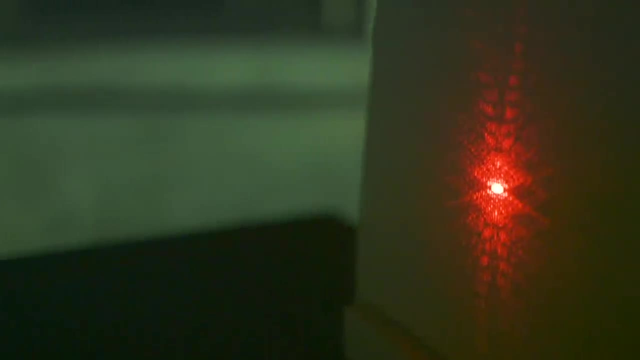 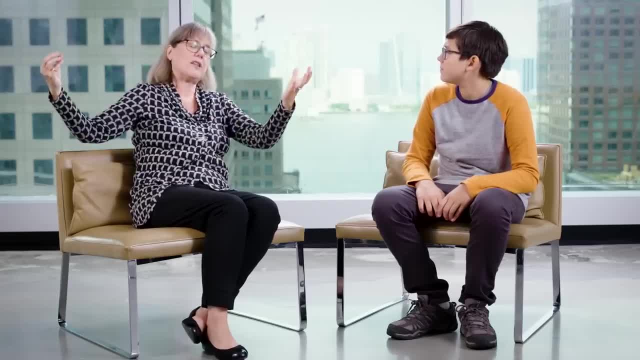 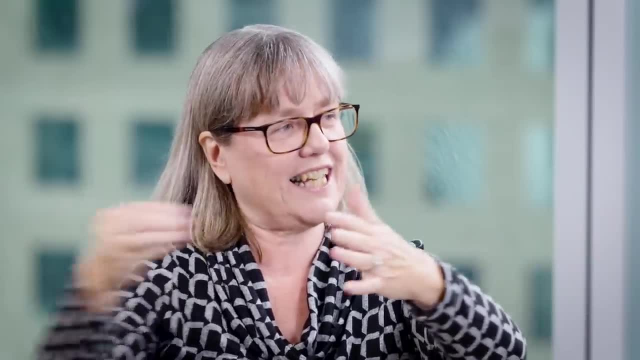 really energetic and sit there for a while, so that when the light comes along it takes that energy and becomes stronger light. And then the mirror sends it back, and it does it again and again and again, And between these two mirrors it makes the light come out in a nice beam, In a laser. 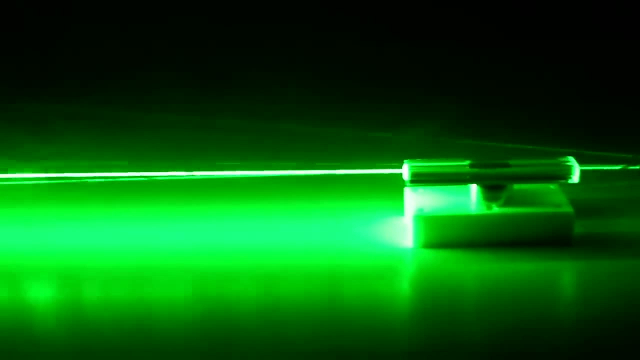 it comes out as a single color. They all come out with their waves at the same time. Every wave peaks at the same time, which then makes the light come out as a single color. They all come out with their waves at the same time, which then makes it a giant wave, And it's this giant wave that has a 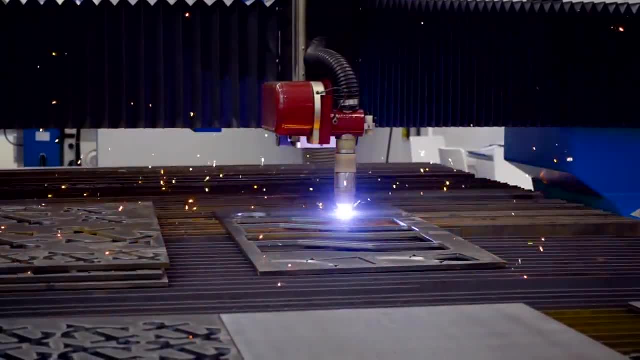 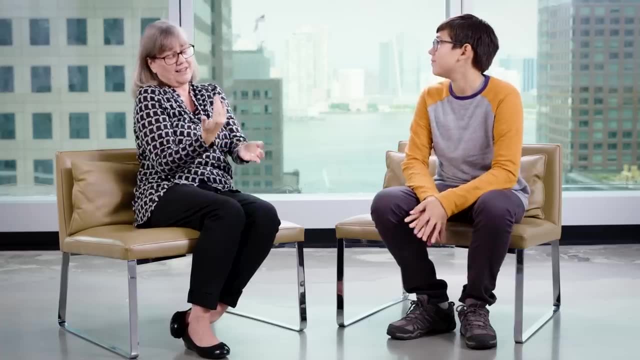 tremendous amount of power so it can do something like cutting steel. But when you cut steel, or if you were cutting this floor, it's gray- It actually will absorb the light. That's why the light you don't see it, because the light isn't bouncing back or through it. 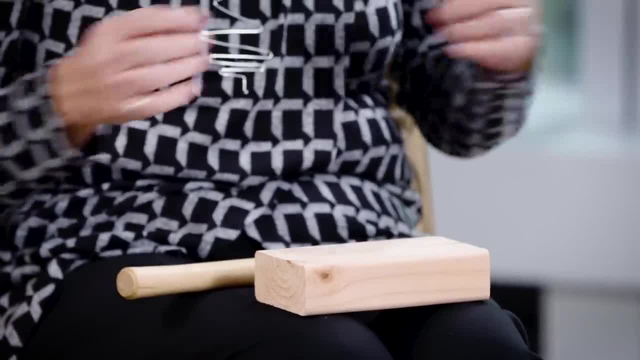 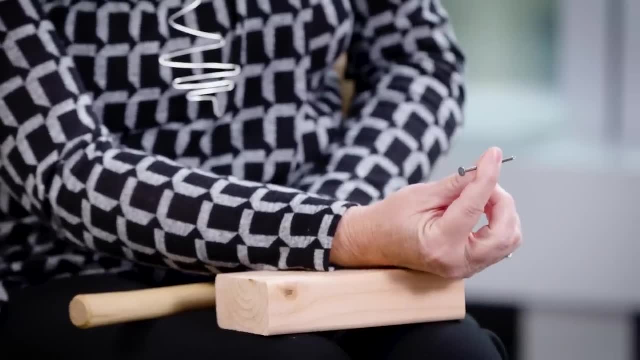 So I like to use demos to explain how my laser works. So I've brought basically a hammer and a nail. I'm sure you've probably hammered a nail before into a piece of wood, but the question is if you asked yourself why it is that we hit the big end. 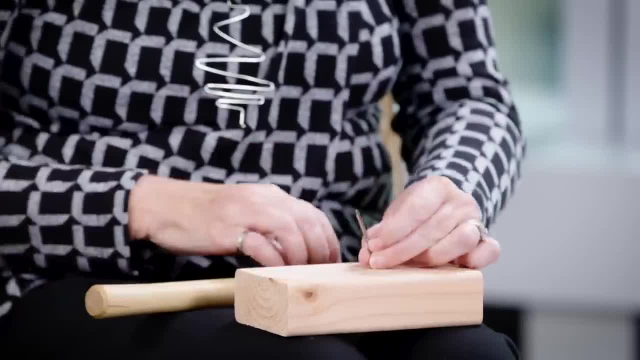 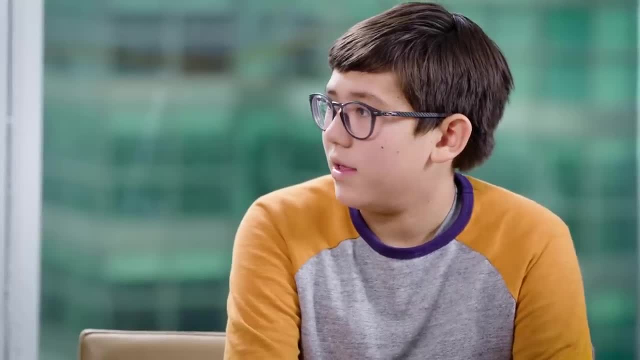 and it's the tiny end that we put on the piece of wood. We would never pick up a hammer and hit the sharp end and hope this would go into the piece of wood Because it needs to be centered so it can more easily just go in. That's right. It's all the same The force that we apply up. 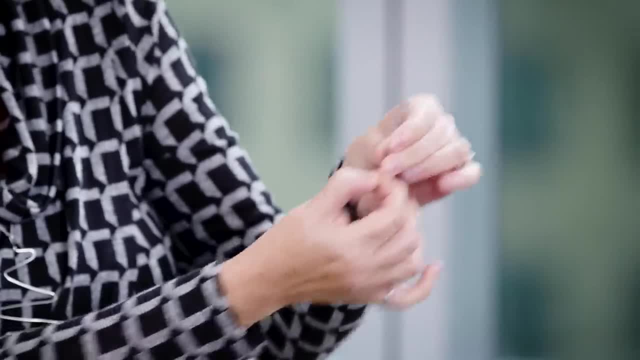 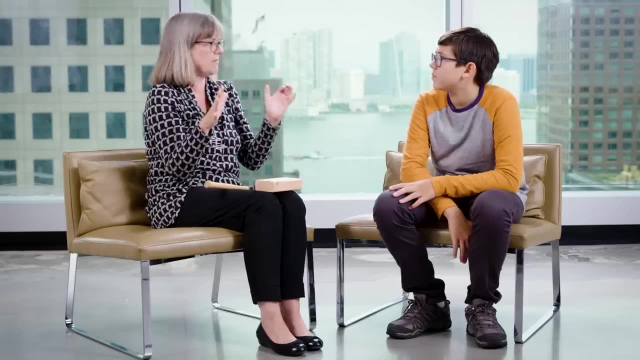 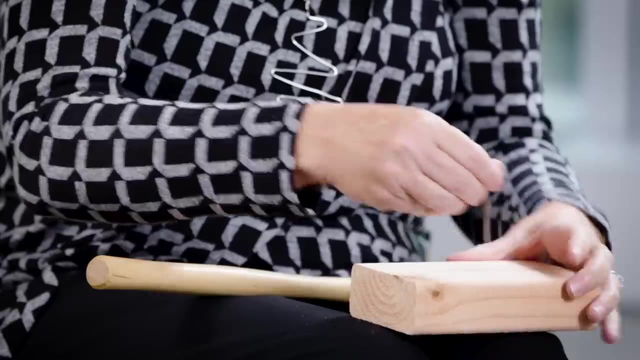 here goes all the way through, but then it can only basically come out when it contacts the wood in that one tiny spot. And so sometimes it's the force that you push something with, but sometimes it is that force per unit area, But sometimes it's not even the force per unit area, because 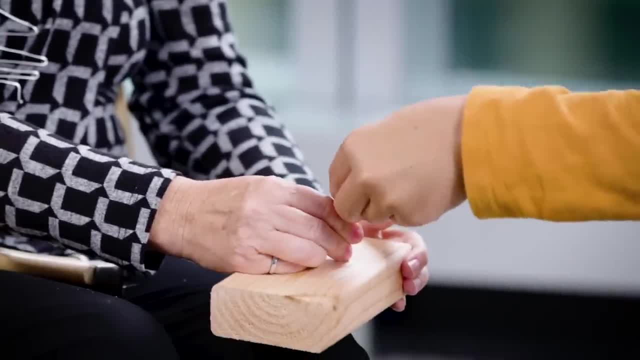 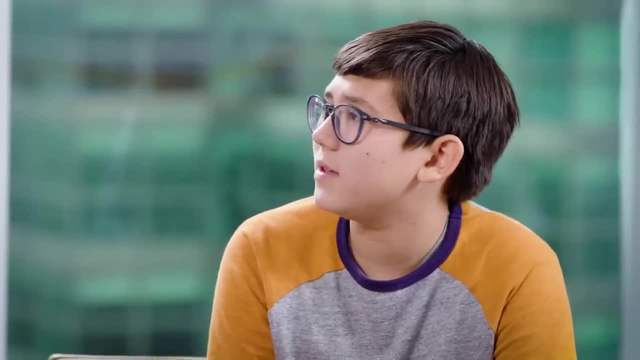 you know, push down as hard as you can on that and see if we can get it pushed in. See, it doesn't really work, does it? So the laser needs all three things: It needs to be centered, It needs time to like, actually penetrate, And then it needs 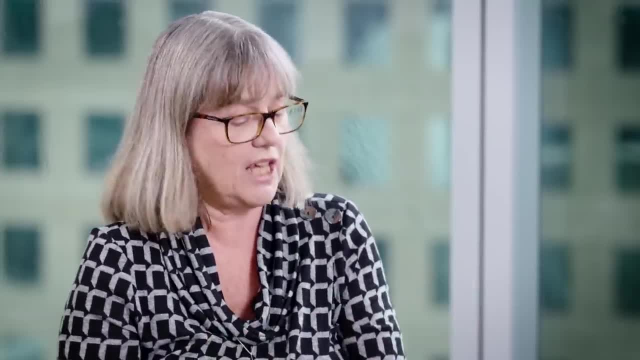 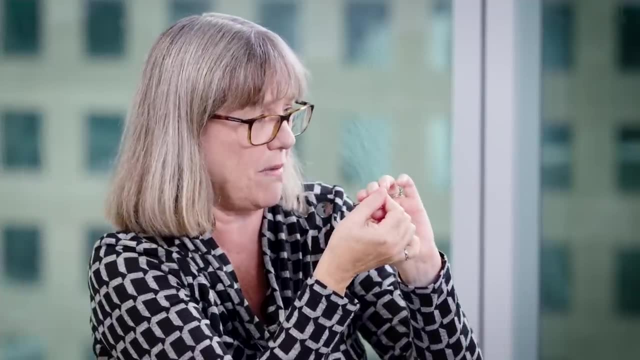 Well, it depends. So if you're cutting steel, you need to have the nail, you need to have it concentrated, all of the light not going in all directions, but you need it into as small a point as possible, and for that we use a lens. for a lens, the light's 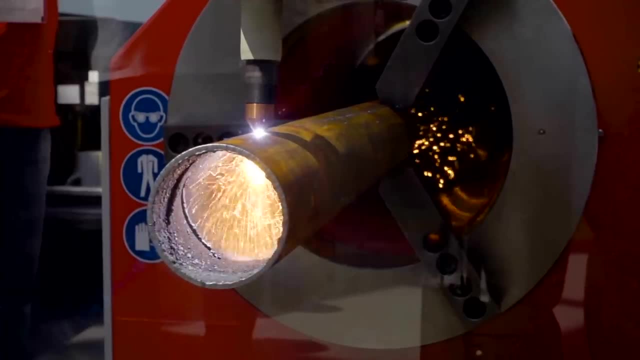 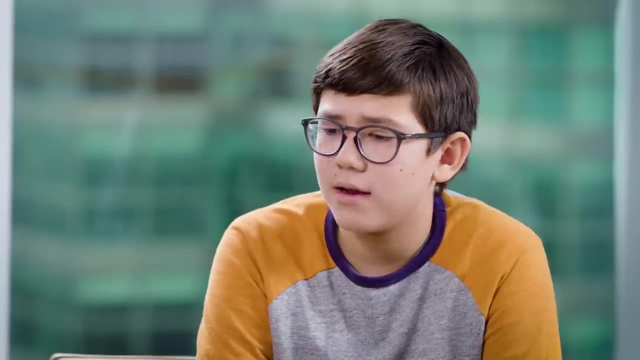 coming down as a column. you put in a lens, it all focuses it down in the same way as the nail and then it starts cutting that steel okay, so that's sort of force per unit area. so it's kind of like a magnifying glass, like it magnifies the light down to a point exactly. you know, sometimes you 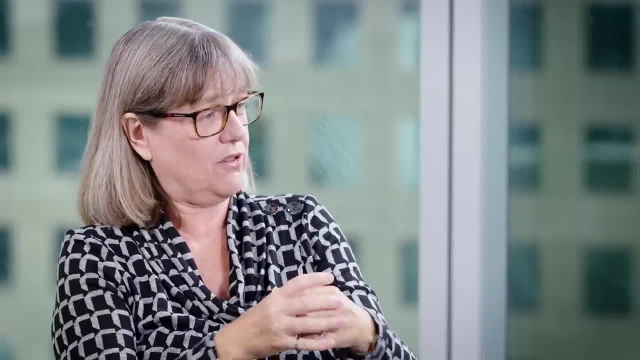 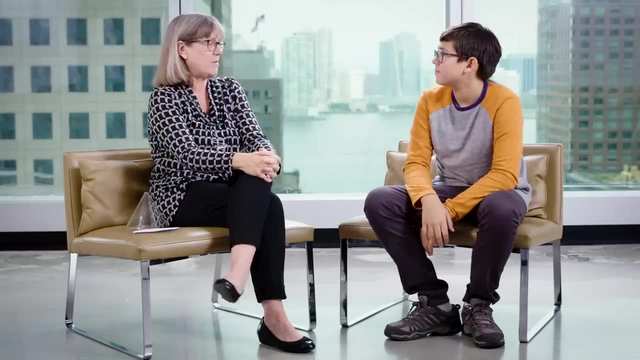 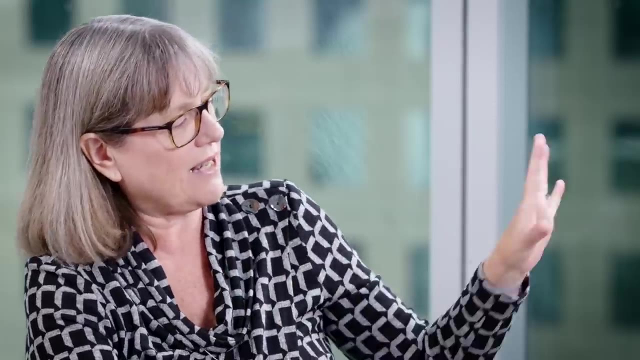 want to have all of your energy, not just in a small area but in this small volume, and so one of the other dimension is time or length. but with light, time and length are the same thing, because light always travels at the speed of light exactly. but if you send a one second long, 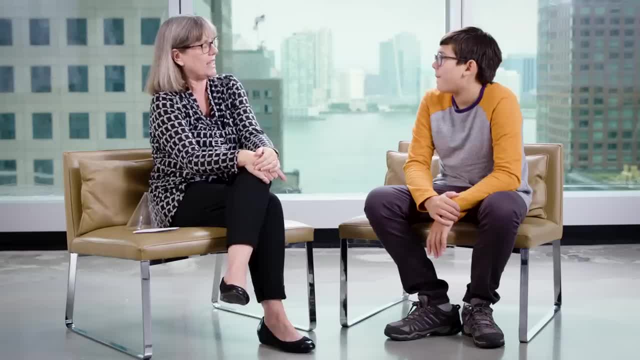 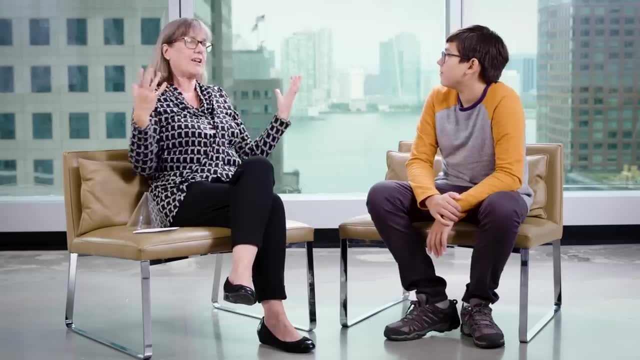 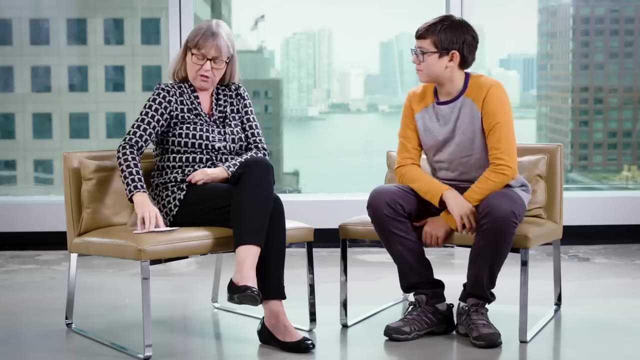 light pulse out into the skies. there the beginning of the pulse is actually two-thirds of the way to the moon. it's 300 000 kilometers long. so now, if you talk about light being concentrated, that doesn't seem very concentrated. the type of lasers i play with in my lab will be no thicker than. 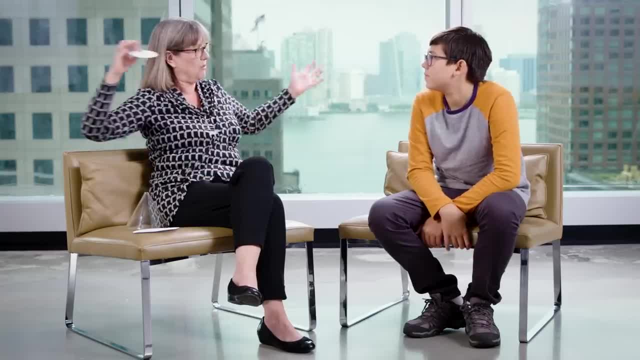 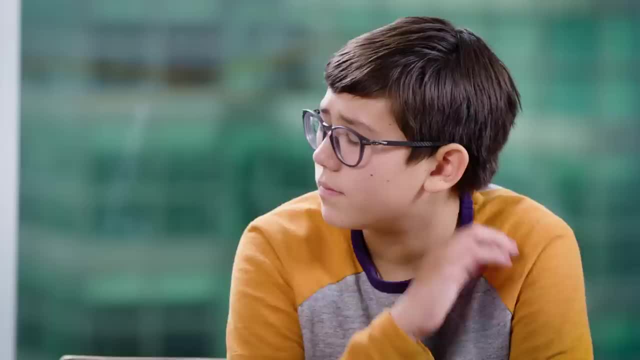 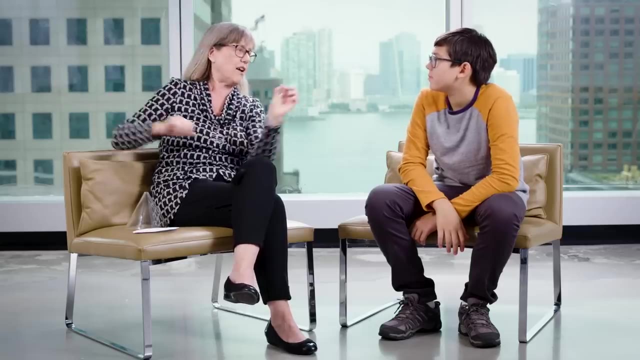 this one piece of paper. so we take that energy that might be in 300 000 kilometers and we squeeze it all the way down into just this piece of paper, and actually the beams are more the size of this piece of paper. okay, and so in my lab they would be flying. pieces of paper like this would be flying through. 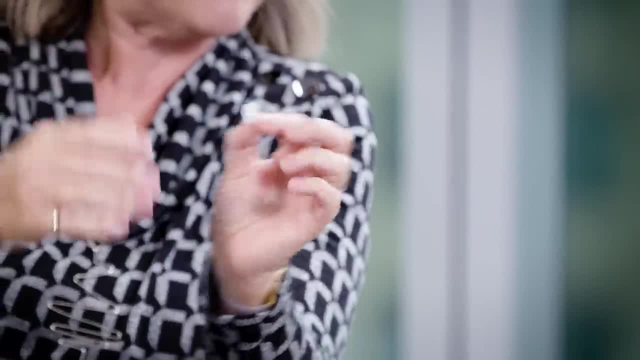 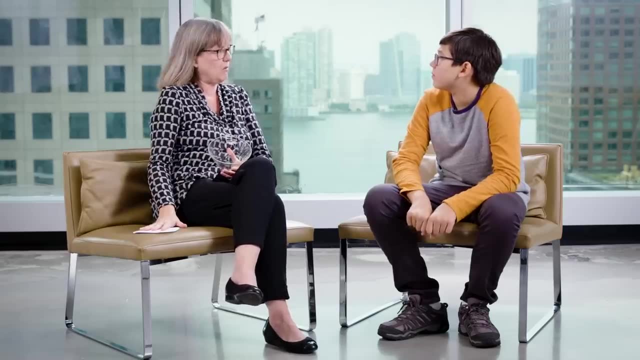 the sky, but we can't see them because they don't come in our eyes. they fly by us and they're infrared. they'd be like little concentrated beams of light exactly everywhere. and so now, if we have light like that that we want a machine with, i bring this funnel, and so if we had a lens here, the light was coming down, so funnels into into a 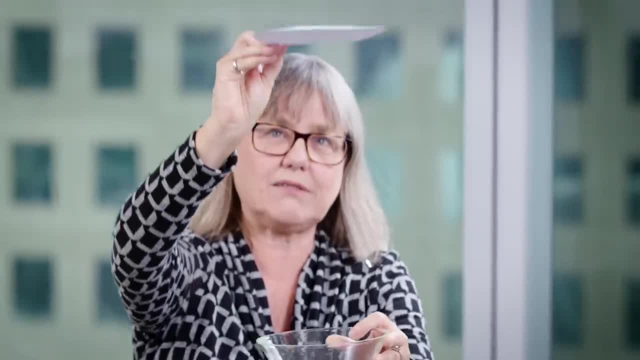 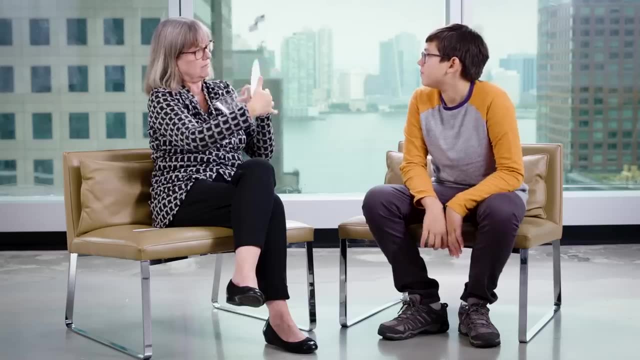 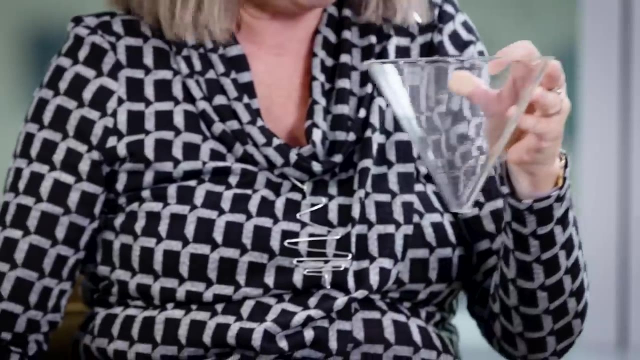 spot. so here would be my light coming from my laser and it would just be coming down, down, down, down, down. hit a lens and we have to focus down, but now all the light started out with this big of a spread, so concentrated this much. eventually it would be here, more concentrated, but by the end, right at the 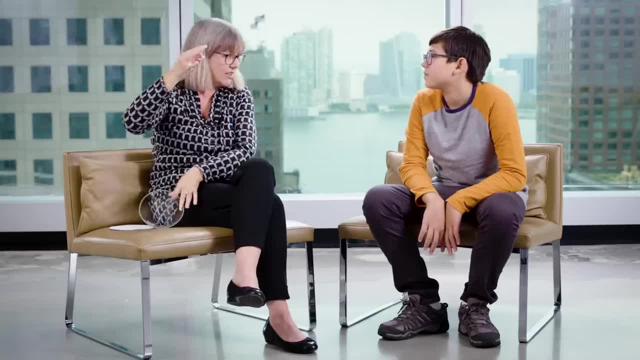 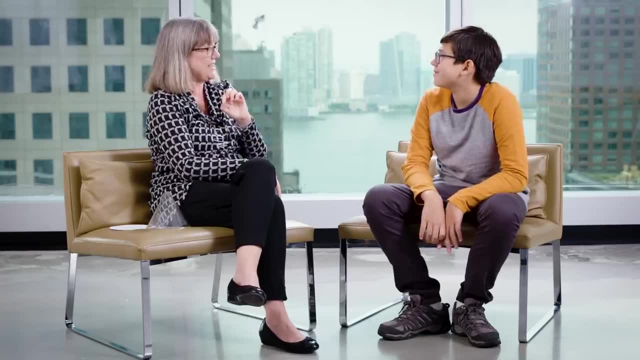 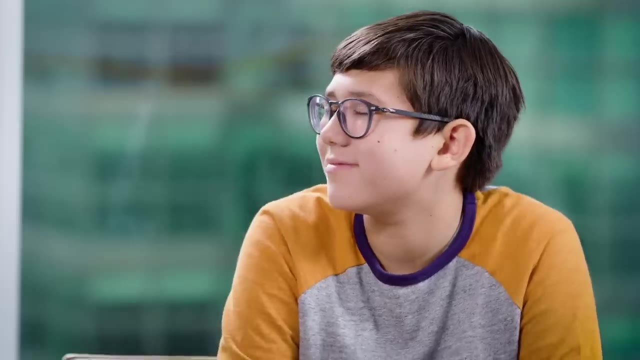 focal spot. that's when i get all of my light. all of the energy has been squeezed down into fitting it inside this piece of paper, and that's why i say that i built a laser hammer, because when this hits a piece of glass, it just smacks those electrons right off the atoms and there's 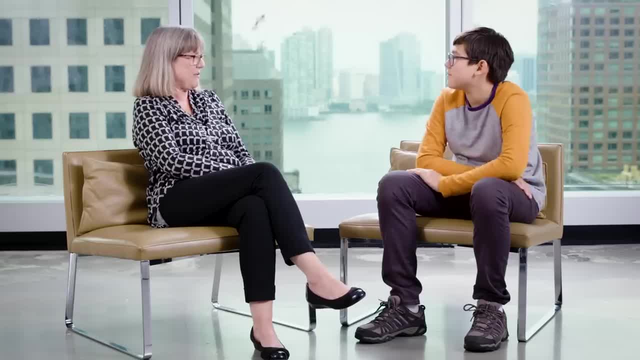 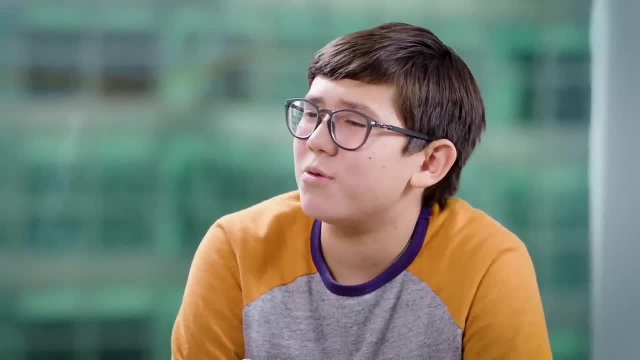 nothing else for them to do, they have to fly away. so can you tell me what you learned, and maybe about the focusing of the light? well, what i learned is lasers. they aren't like particles, they're more like a super concentrated beam of light that can be any color they get. really. 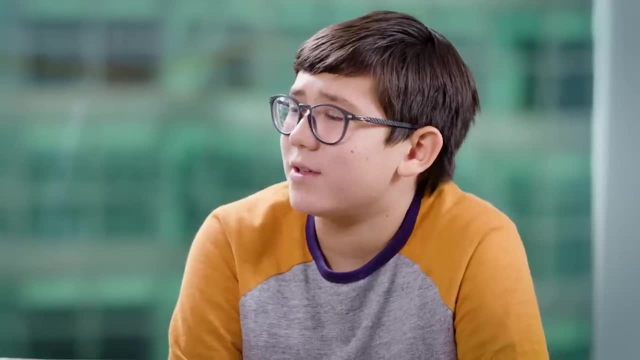 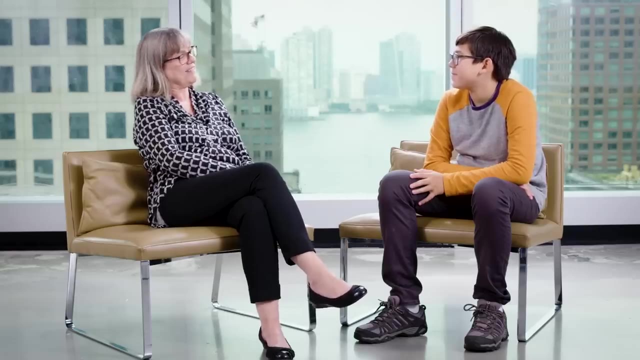 concentrated, and that's what makes them like blazers, and that's why they concentrate things and break things, because it just moves the electrons out of the way. so do you think that lasers are fun enough to talk with your friends about her? of course i'm going to have to share. 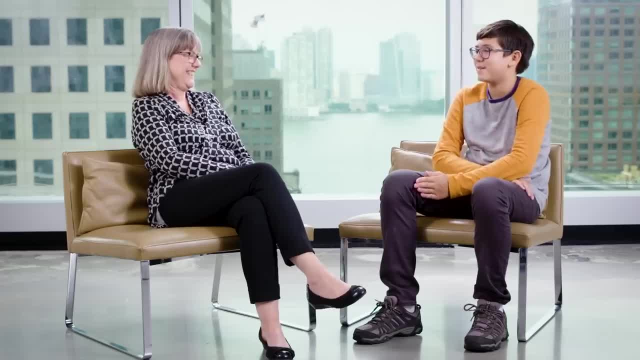 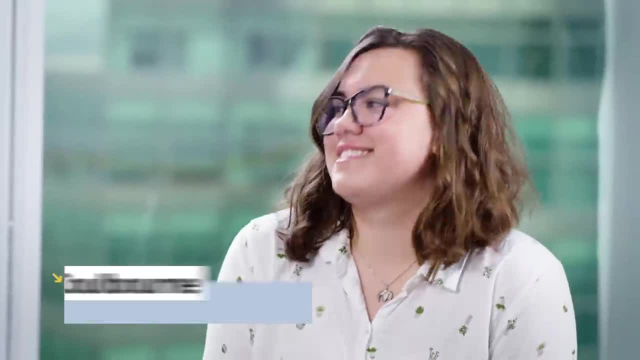 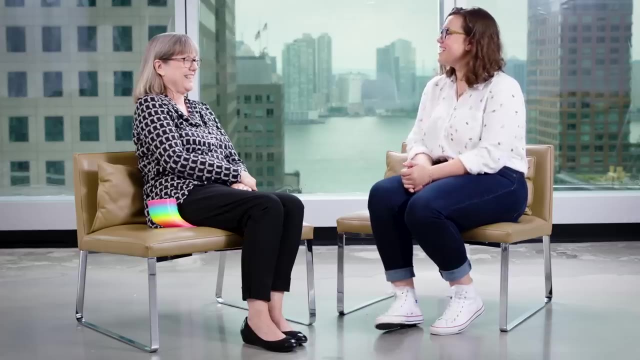 something about my experience learning about lasers with an expert like you. so you're a college student, yes, and what's your major? um, i'm an engineering physics major with a minor in math. i'm in the 3-2 program for biomedical engineering. excellent, i got an engineering physics degree. there you go something. 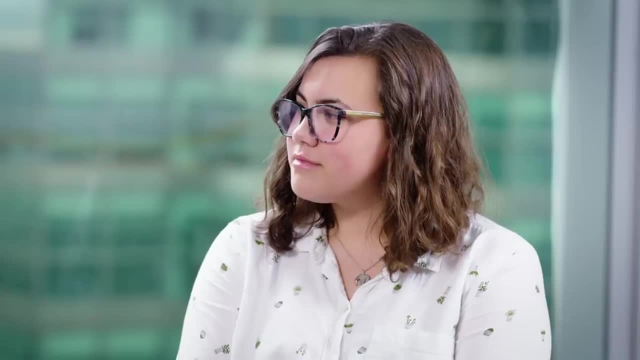 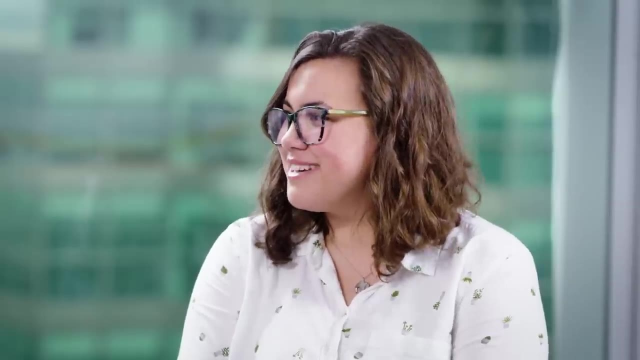 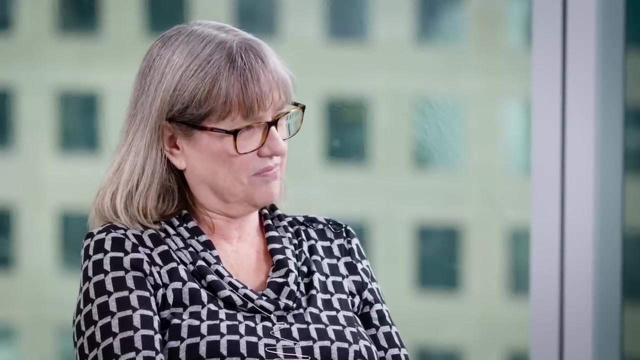 common. we're here today talking about lasers. so have you had much exposure to lasers yet at school? not yet. um, i i'm really hoping that we will. uh, i think it's super interesting- just the field in general- because i really do enjoy examining all the calculations and being able to do a little bit more of the math side of physics. 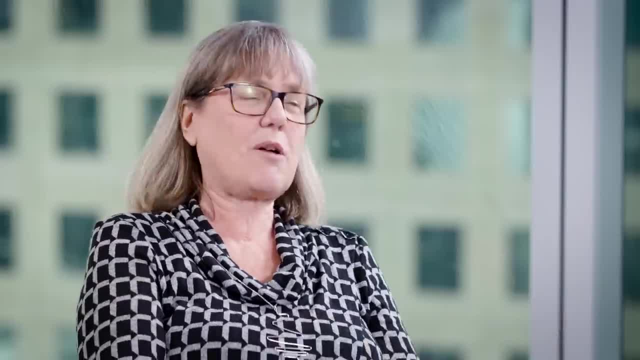 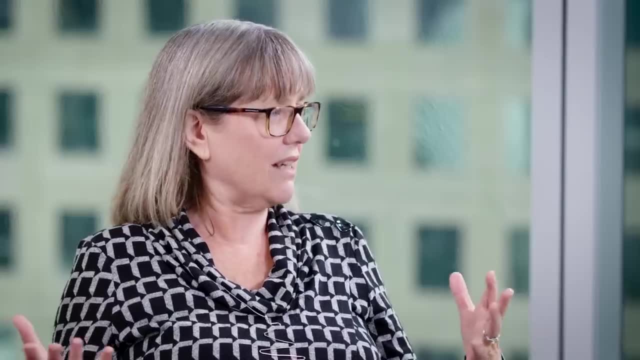 okay, as opposed to the experimental side of it and seeing things okay. so i'm much more. i like to see the things happening. so then the question is: what's so special about making a light that's intense enough to actually possibly blow things up? Certainly, we can blow atoms up with the laser hammer. 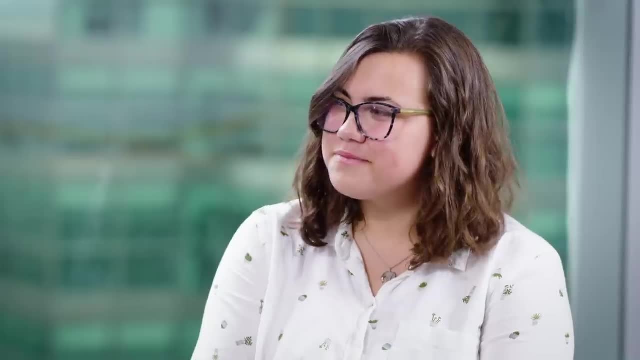 and the laser light comes in and just smacks the electron right off the atom, And so the question really is is: how do you make that Back in the 70s and into the 80s? I know that's a long time ago for you. 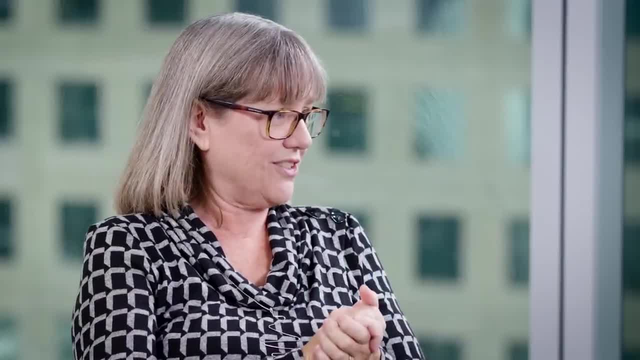 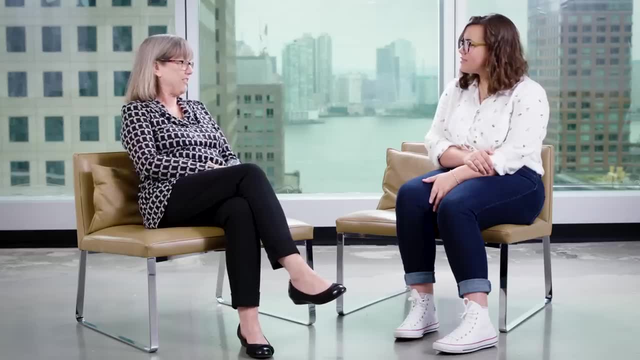 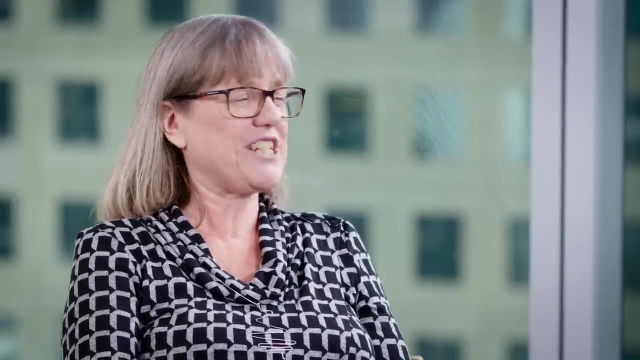 we had big energy lasers and we had short pulse lasers. We couldn't have big energy short pulse lasers And actually it was my supervisor and I that figured the way around that and we got something called chirped pulse amplification. Have you heard of chirped pulse amplification? by any chance? 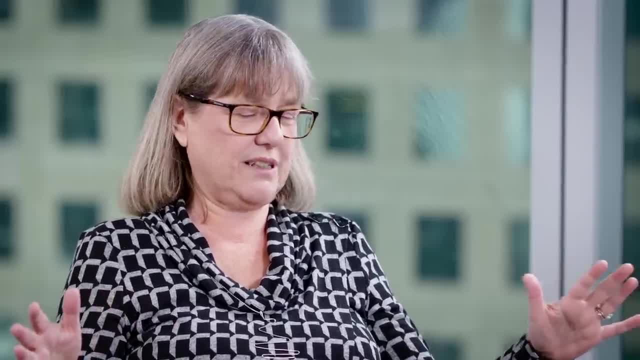 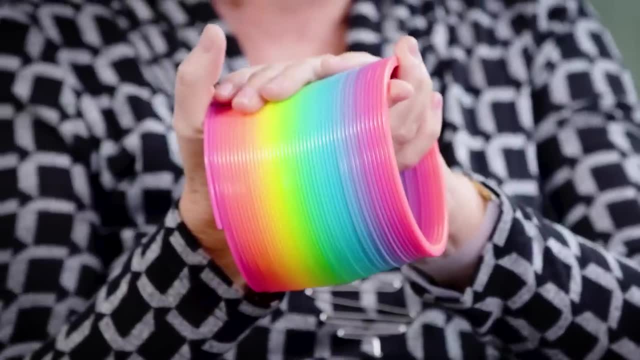 Vaguely. Well, I brought a little bit of a prop to explain how chirped pulse amplification works. Our short pulses are made of different colors. I've got a colored slinky here. We probably could have called it stretched pulse amplification, but that's kind of boring. 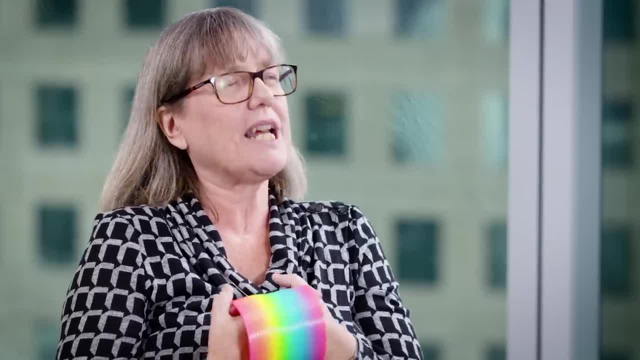 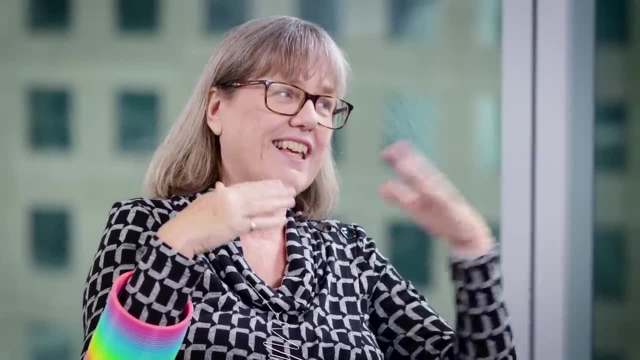 So we used the word chirped. The word chirped comes around because birds chirp. When the birds are singing, the notes are actually changing audio frequency with time, And that's a chirp. The point is that when all the light is squeezed together like this, 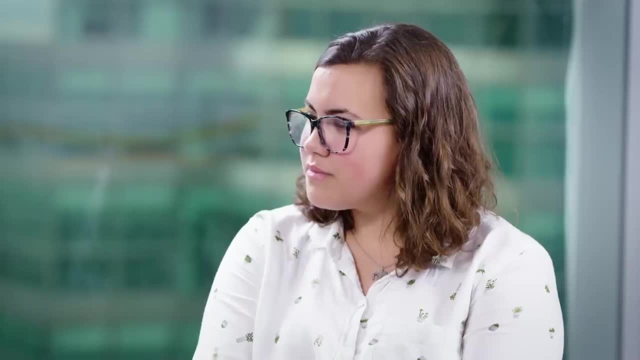 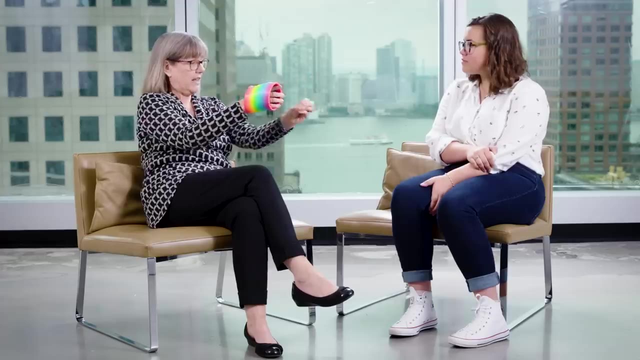 it's a short pulse and that's when it's a hammer, because all the light is now concentrated. And you can imagine if this was coming along and also using a lens to focus it small, then all of that light at the focal spot concentrate. 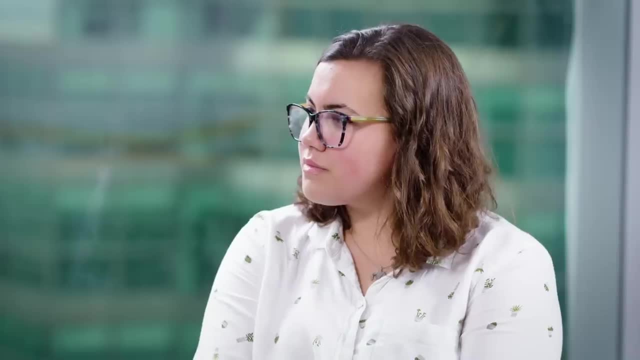 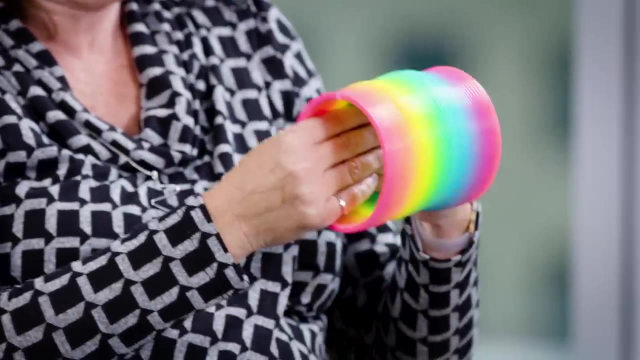 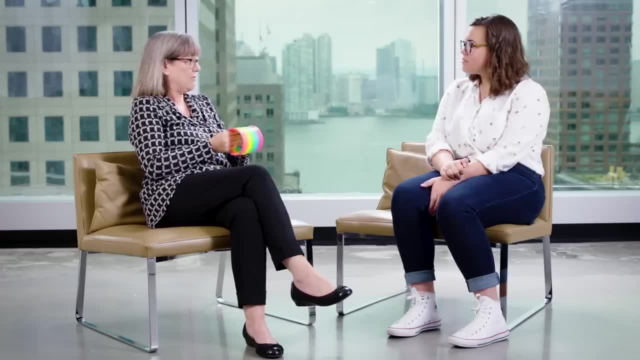 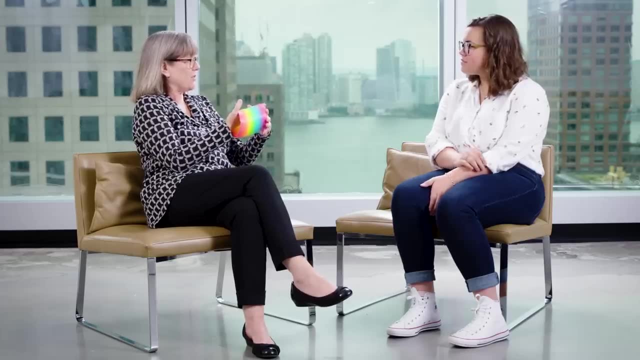 Inside material. So we used a long fiber, 1.4 kilometers of fiber. but in fiber the red colors really haven't got that much in common with the glass atoms And so they spend very little time, you know, interacting, and they travel fast. 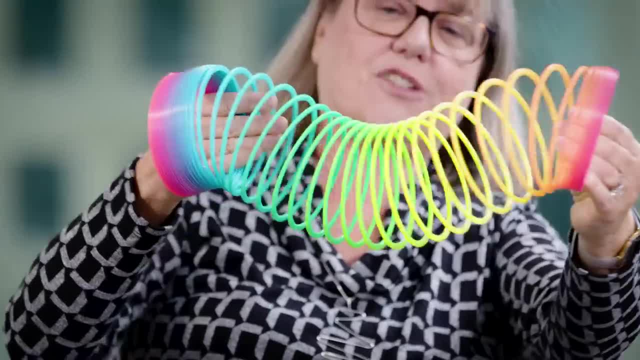 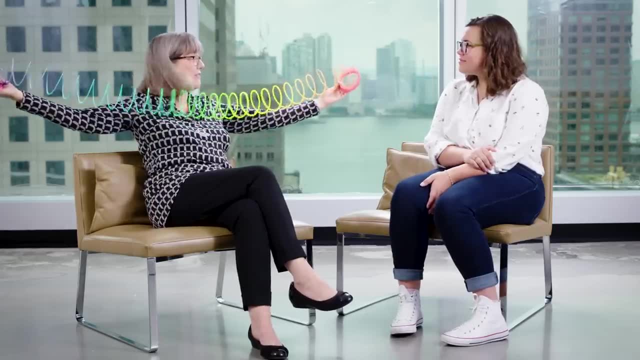 The red is going to start traveling, faster than the green, faster than the blue, And as you travel down the fiber, next thing you know you have a long pulse and it's chirped from red at the beginning to blue at the back. 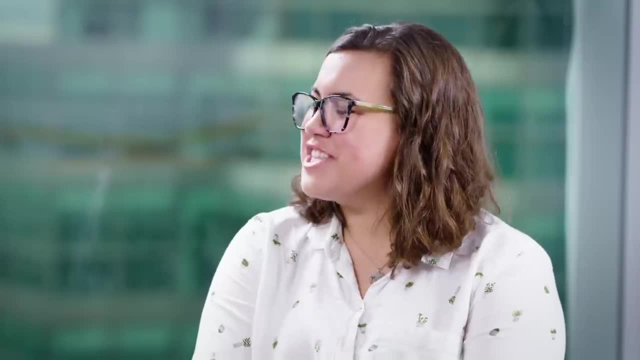 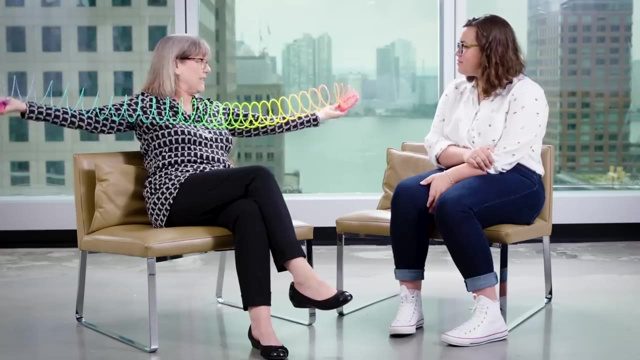 And so the frequencies go whoop like this. So this is a chirped pulse, and now it's a long pulse. And so first this is what we did: we chirped it, we stretched it, then we can safely amplify. 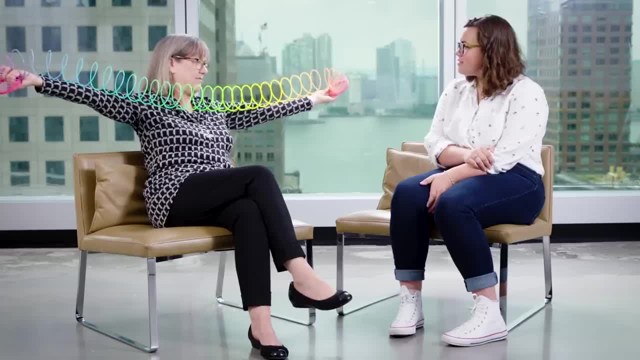 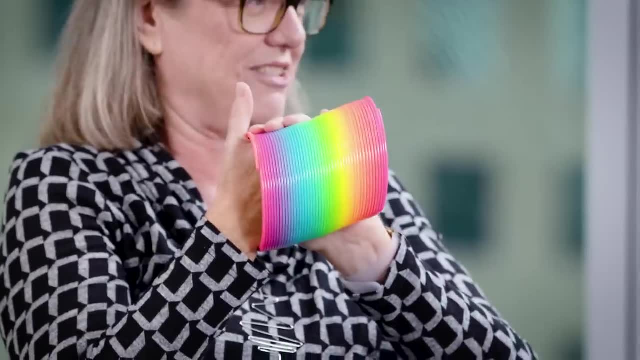 it because it's not all concentrated, And after we amplify it, then we use something called a compressor and we put all of the colors back together and it was back being a short pulse but a high-energy pulse, And together then we really had what I like to call a laser hammer. 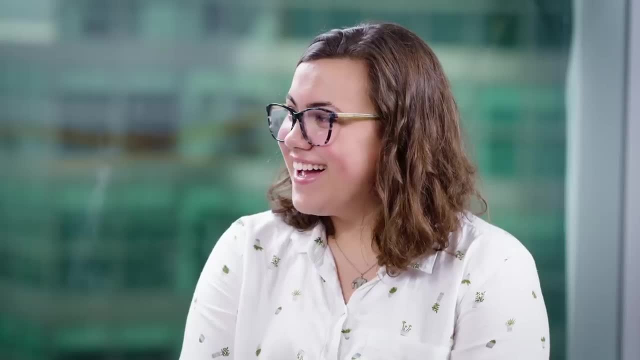 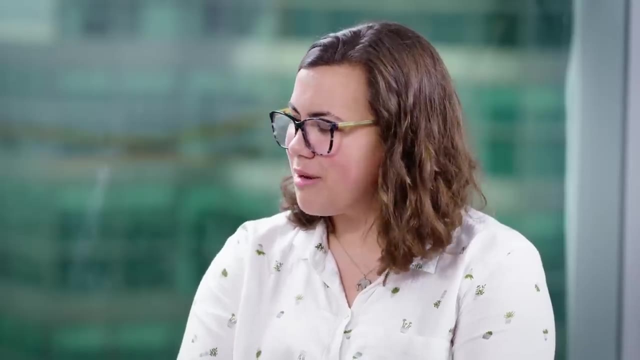 When this laser pulse goes inside, it smacks those electrons right off the atom. So the laser hammer that you were describing with other types of lasers and the one in the chirped, is it still the same premise? Well, a lot of lasers, and when lasers first came along, they were only single color. 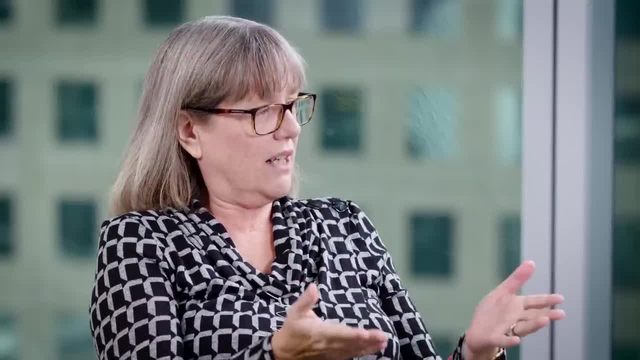 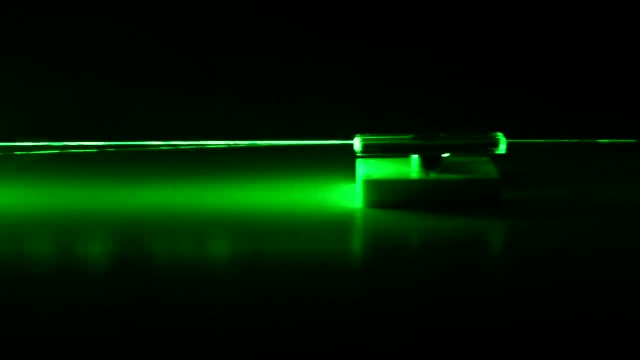 Your cat toy will only be a single color, probably a red one, and so that's just one color. And one color means that it has to really be there for the whole time. One color is one wavelength of light, and so it's just one wave that goes on and on. 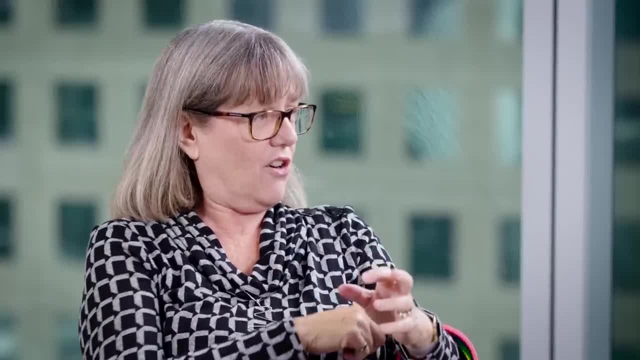 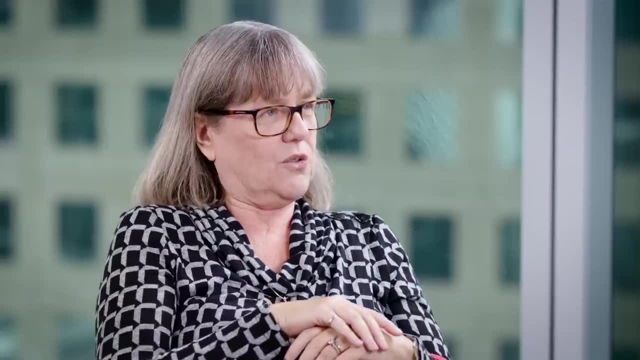 and on. If you want a short pulse, you actually have to have all the colors and if you can imagine at one point, One time, And I like to say it's like a conductor of an orchestra, When you're listening to an orchestra, warm up, they sound terrible, they're all playing. 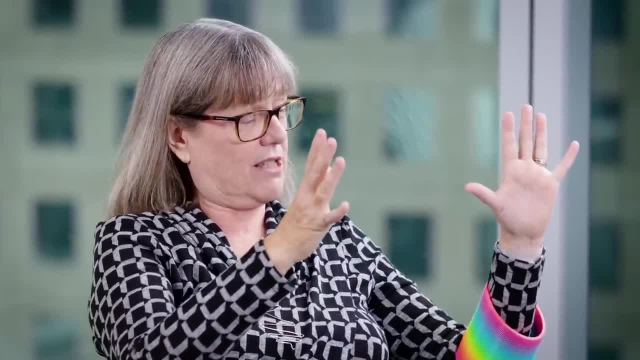 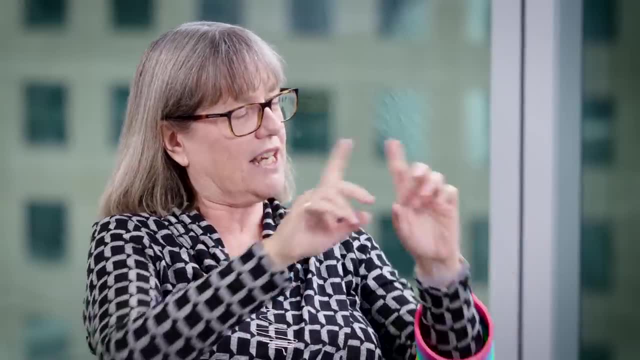 their own notes, but when the conductor conducts them they all play different notes, but together it's beautiful music. So we have something in a laser called a MoBlocker and it's like the conductor And it says: go now. 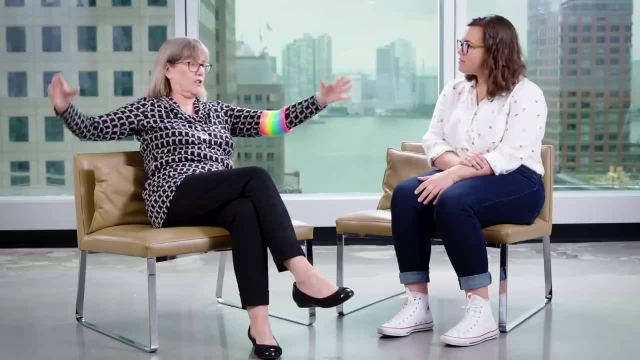 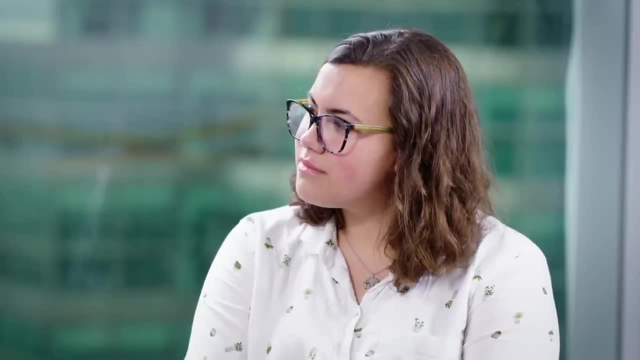 And all the colors will start together. but some colors are long wavelength and others are shorter. So next thing, you know, you have peaks meeting valleys and they cancel each other, And so the more colors you can bring in, the faster that happens and the shorter the. 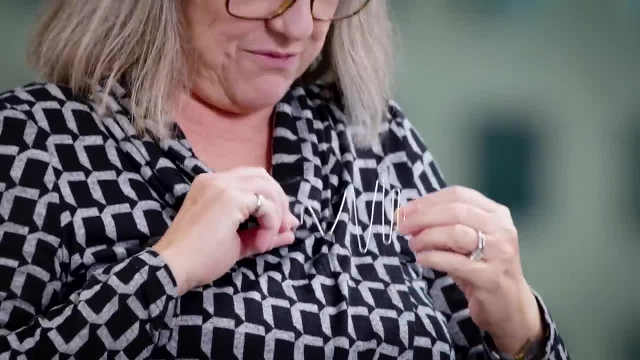 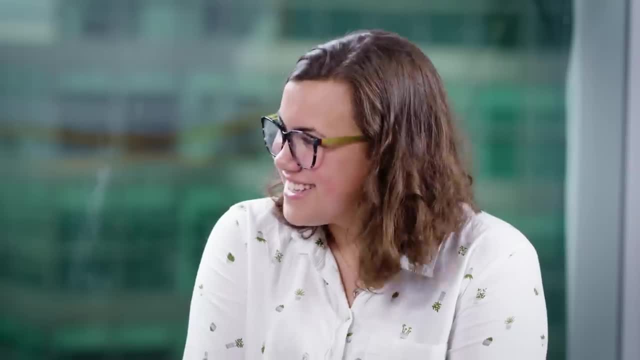 pulse you can make. The necklace is something that was designed for my Nobel Prize. It's sold at the Nobel Museum and it is a chirped pulse. So we've been talking a lot about lasers and applications. What have you learned about chirped pulses? 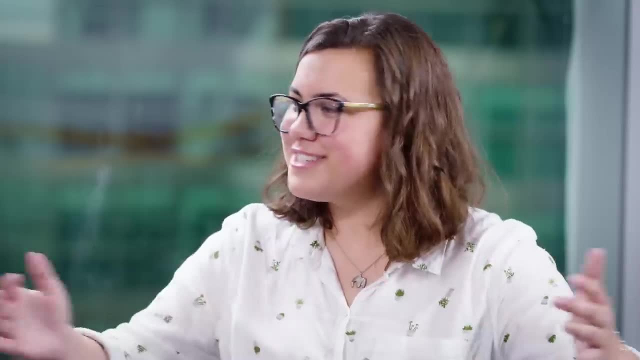 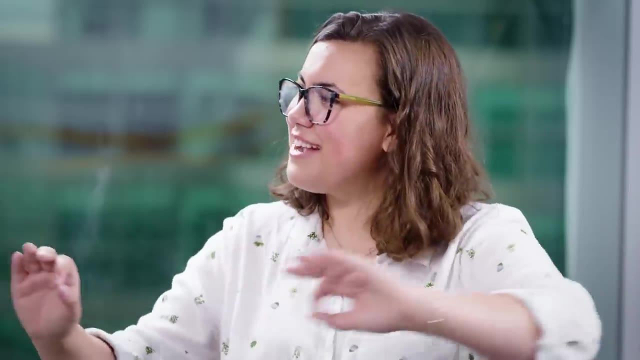 I learned that it all stretches, which is super cool because red moves the fastest and so it kind of tugs around. But it's not just the pulse, It's the pulse, It's the blue. It really threw me off just how fast. 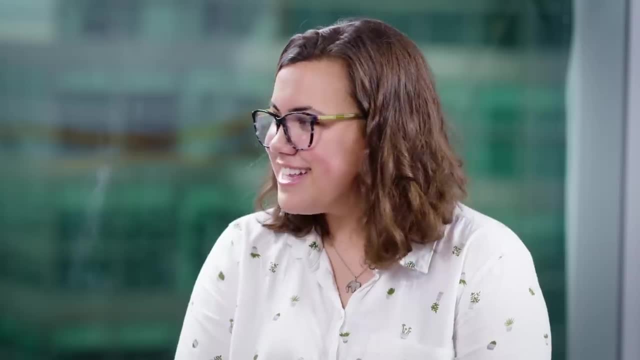 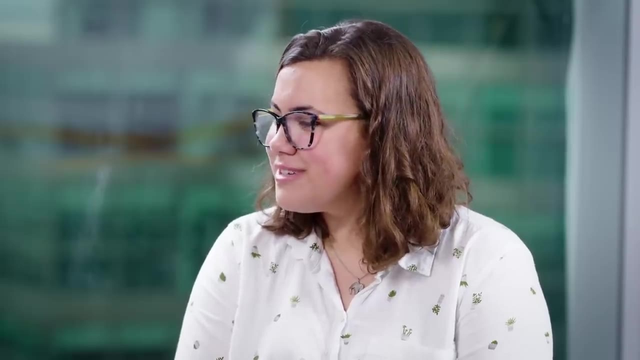 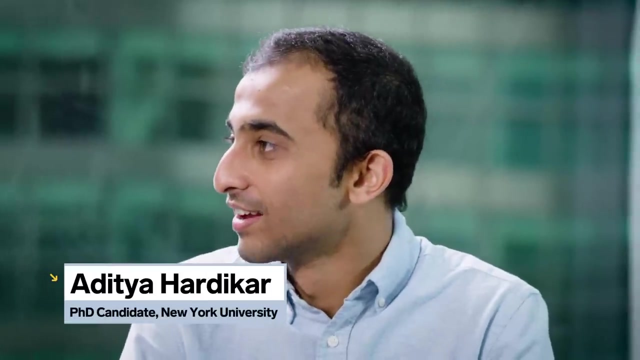 It's hard to imagine things happening that fast, And I also learned how many of the things that I know are lasers and how many of the things that I've been looking for, like the answers to it, is in lasers. So I understand you're in grad school. 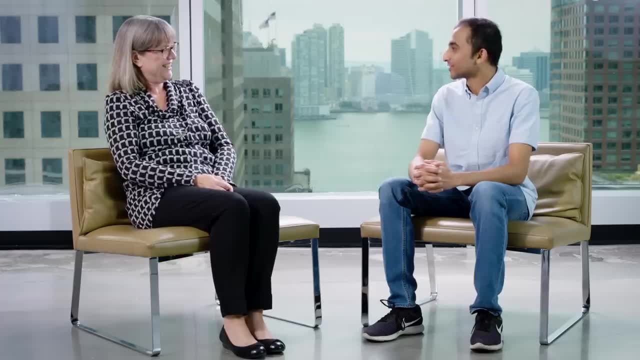 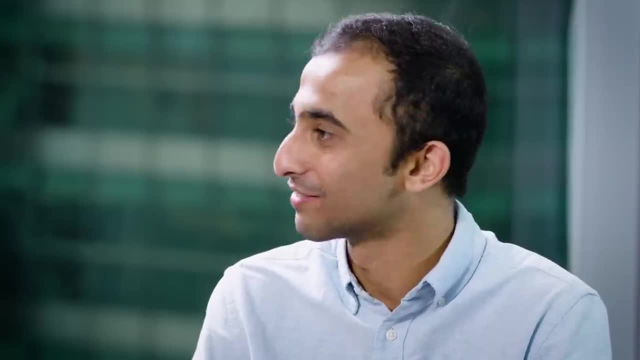 Where At NYU? And what are you studying? I'm studying soft matter physics, which involves the physics of squishy stuff. So we have a lot of pro swimmers in the laboratory and we drive them with a laser. And what kind of laser do you use? 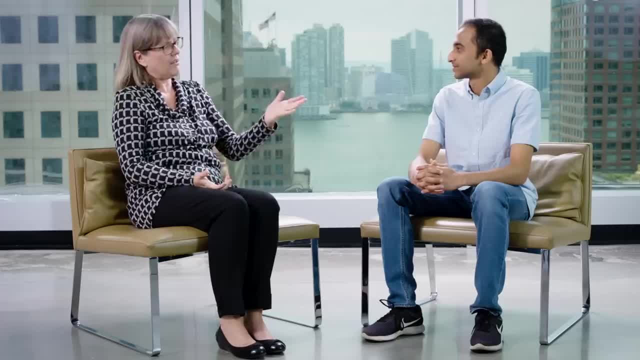 We use a 10-watt laser. It's a fiber laser. Do you know a lot about lasers, or just about the laser that you use? Not a lot, Just a little bit. OK, So this is about high-intensity lasers. 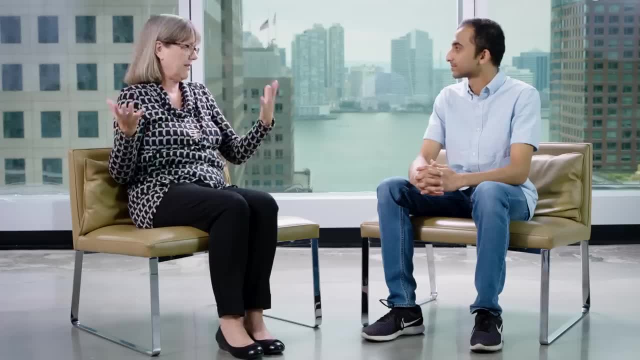 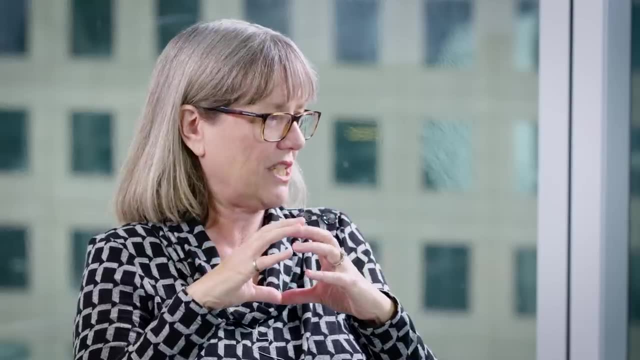 OK, Not only how do you make them, but what was really stopping them being made? In both cases, it's nonlinear optics. OK, You know we want to do something that requires a huge photon density application. Yes, And so that's how come we came up with chirped pulse amplifiers. 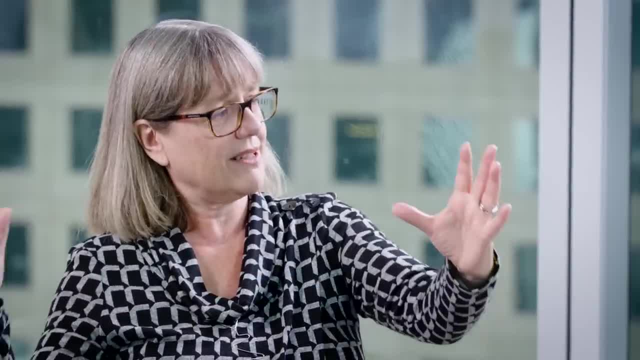 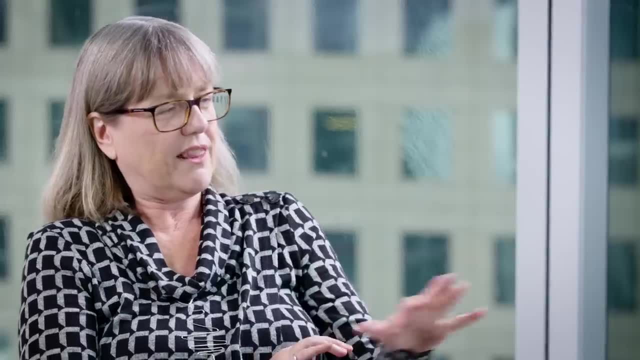 OK, So we have a chirped pulse amplification so that we could stretch the pulse safely, amplify it, then compress it at the end, and then we're ready to do whatever we want at the end. So what do you think the main difference is between the continuous wave laser that you have that runs at 10 watts and a chirped pulse amplifier. I feel like the continuous laser delivers power at a continuous rate, whereas you want all that power to be delivered in a really, really short time with your amplification, And so we get the power with a lot less power. Right, And so we get the power with a lot less energy, because it powers energy per unit time, Right, So we aren't depositing much energy in comparison. Yes, Can I just ask? Sure, Because you are using the thermal process of it heating up. 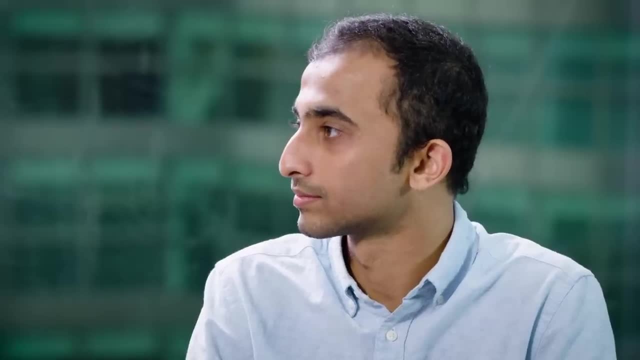 Yes, But have you ever had the opportunity to use laser tweezers? I have, yeah, We use optical tweezers to trap particles in a solution. OK, And twirl the motors or not. twirl the motors, No. 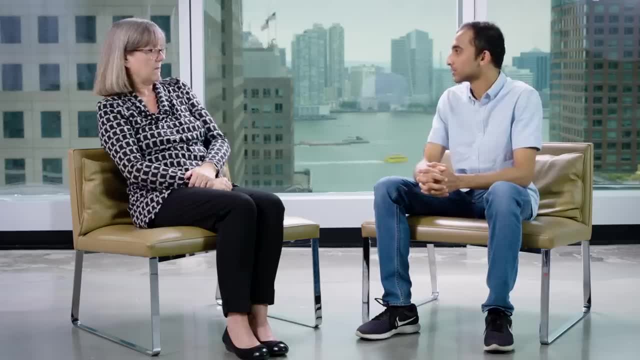 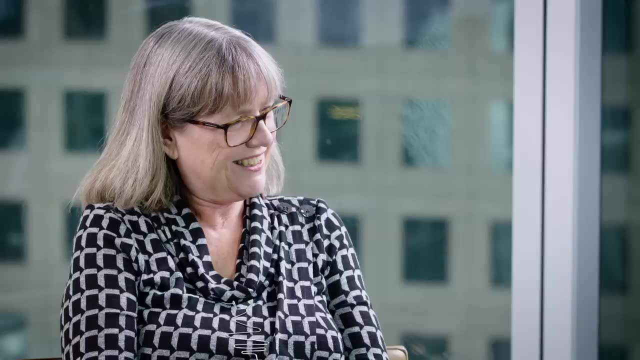 I haven't worked with that, You haven't OK. So I was always curious: how much further, like what higher power, can we go now? So chirped pulse amplification took us sort of from we were at 10 to the 12, but when 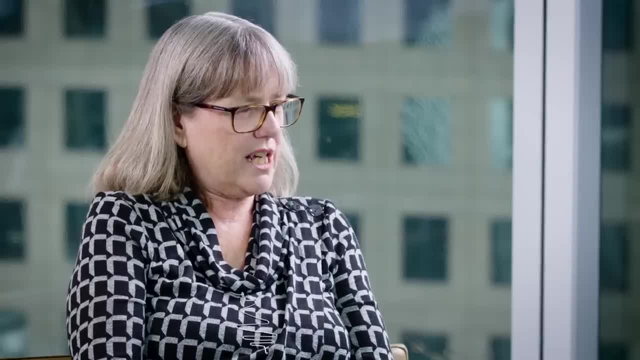 I was working the 10 to the 12 sort of sat on a football-sized field. It was a kilojoule laser with a nanosecond pulse, OK, And we brought it down to something we call tabletop terawatt. 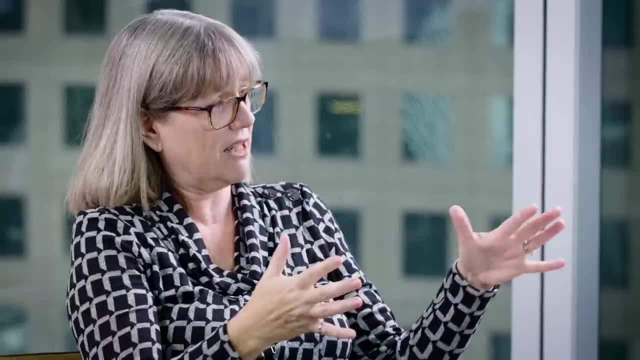 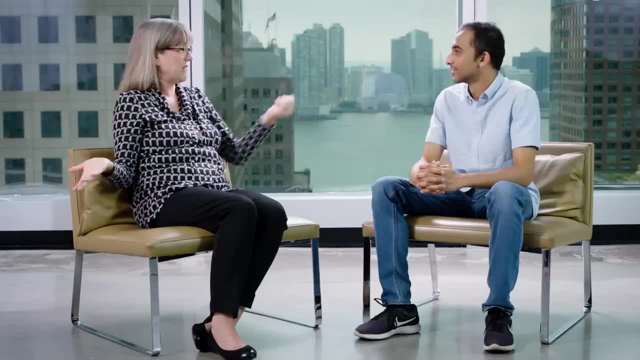 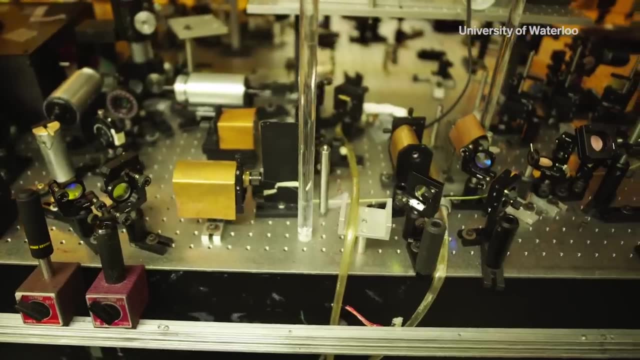 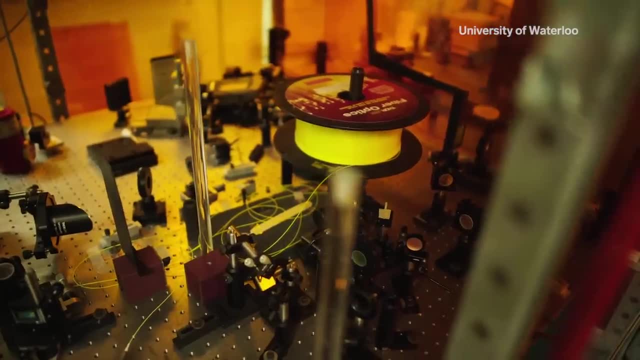 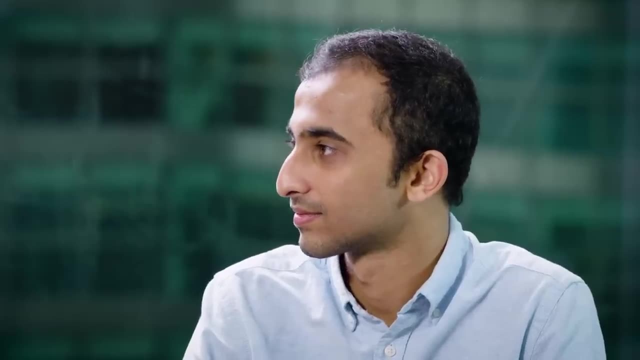 So then, and going forward, one of the holy grails is: can we reach 10 to the 29 watts per square centimeter? So we still have six orders, So we've gone from 10 to the 12 to 10 to the 23.. 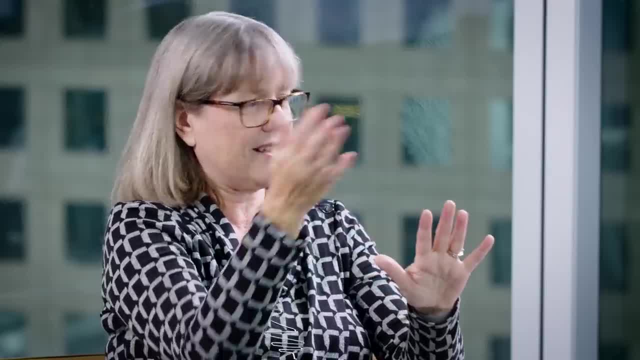 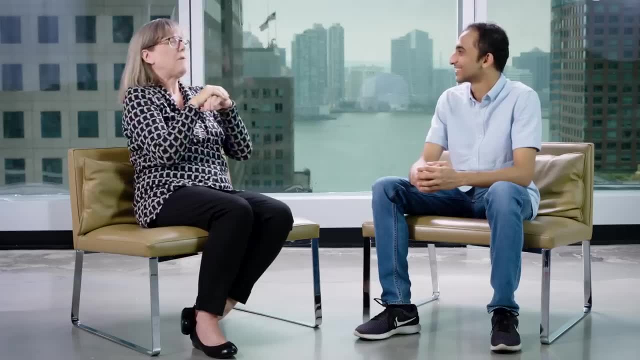 So we've done. you know, 11 orders, So you think six isn't so much harder. I have to tell you, over time it's rolling over, It's. It's a prize-winning idea, But if we get out there, that's where, if you focus the intensity, the energy in that, 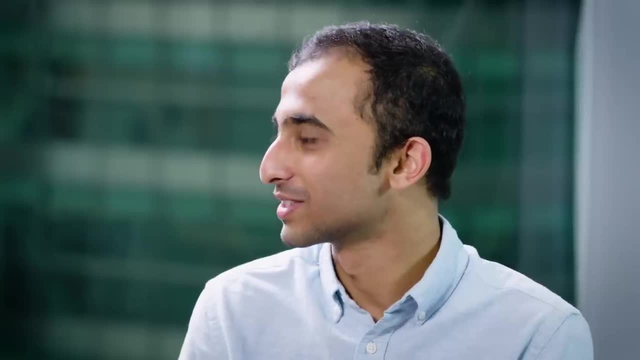 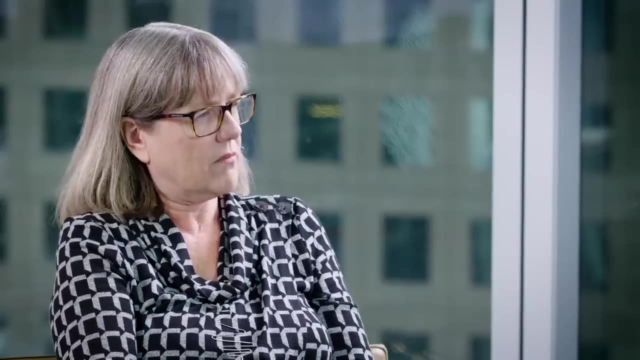 volume is enough to break the vacuum. We could probably use this to drive chemical reactions at a very, very specific spot, like if we want to target just a single cell in the body. Yes, And maybe what do pump, probe, spectroscopy and watch the cell, or to ionize it. I mean, I was thinking more on the lines of if we want to, let's say, destroy one cell like a tumor cell or something, Okay, So that the neighboring areas are not affected, but just the cell burns. I don't know of people working on that because I'm not so much in the medical field. 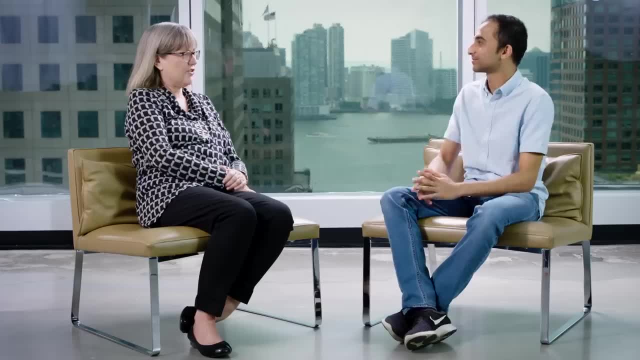 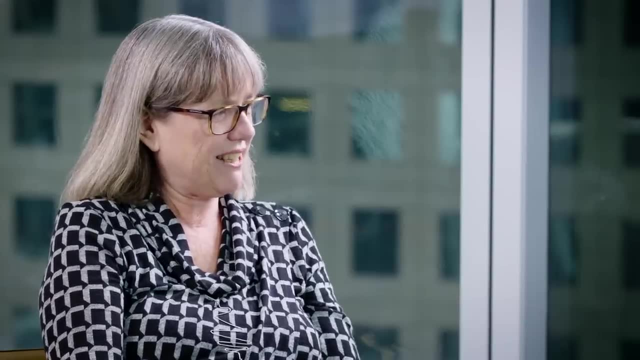 Okay, But I should look into that and see if that's a possibility. So, after hearing about high-intensity lasers, can you think about next time you go back to the lab and you're wondering how to do something in the lab with lasers, can you? 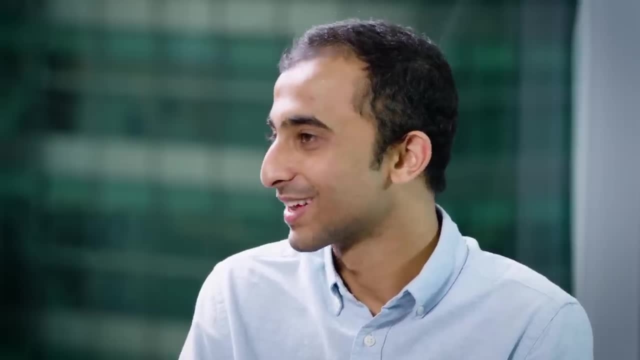 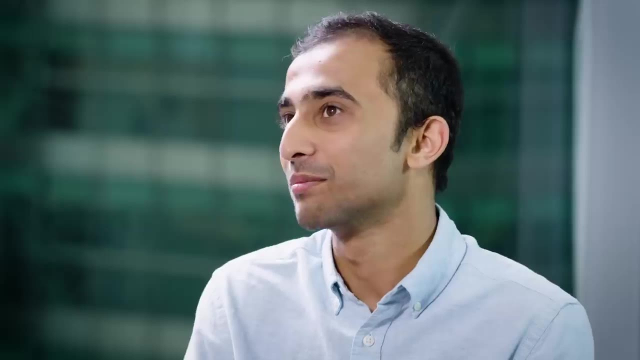 see how short pulses might help you. I think short pulses might help in my experiment in the sense that if I drive my swimmers with a continuous wave as opposed to, Maybe a continuous wave would heat up the sample too much and a pulsed laser would. 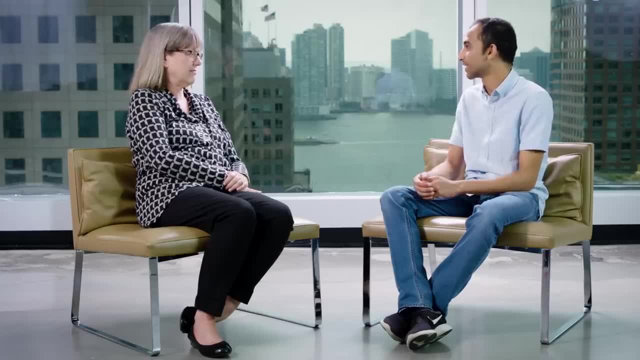 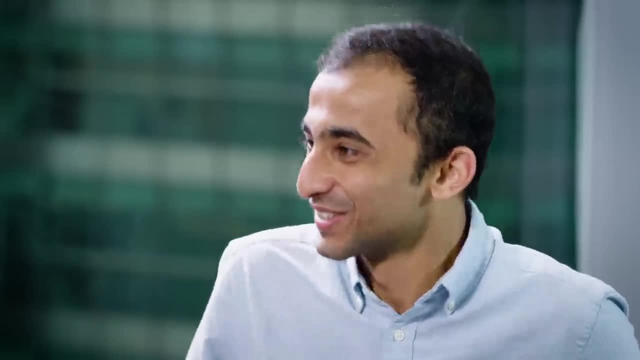 deliver power exactly where I need it, so that I could run my experiment longer. Maybe That's true. Thank you very much. Thank you, Donna. That was good talking to you. It was really nice to meet you. Hello, Donna. 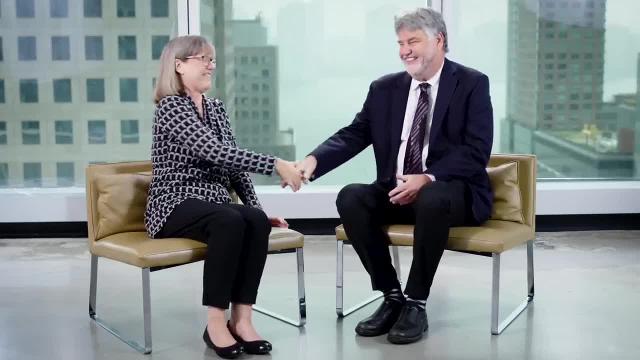 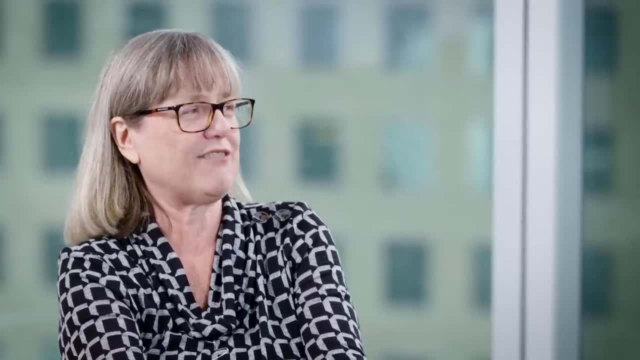 Good to see you. Good to see you, Mike, Nice to have you here with me. So we go way back 1991, the year I got married. I moved across the globe- Okay, I moved across the country, left my husband in New Jersey to work with you in Livermore. 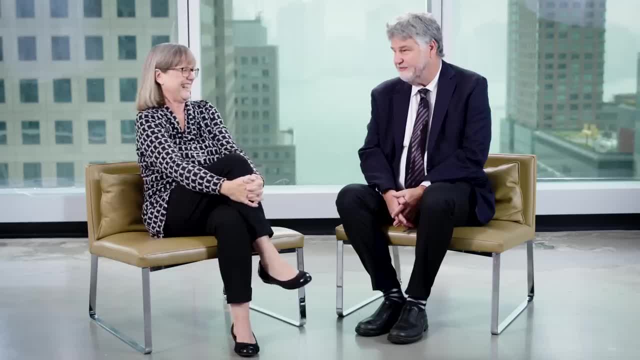 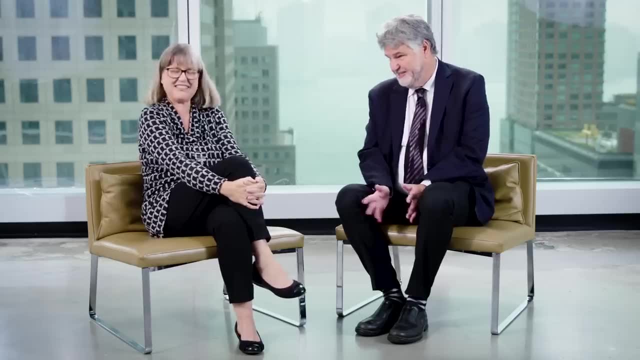 I remember very much how hard it was to convince you to travel across the country and work at the lab And stay there, And stay there. I couldn't convince you to stay, You could not convince me to stay, no, But you were there long enough to make a big impression and get some good work done. 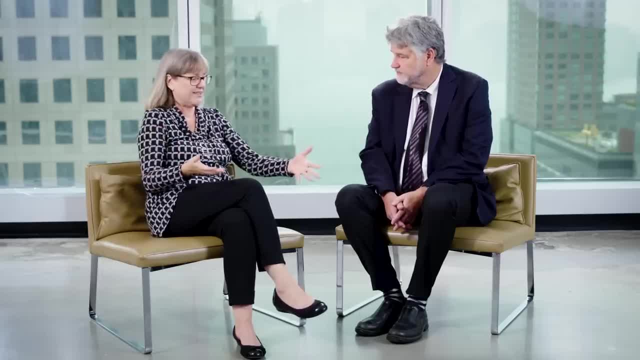 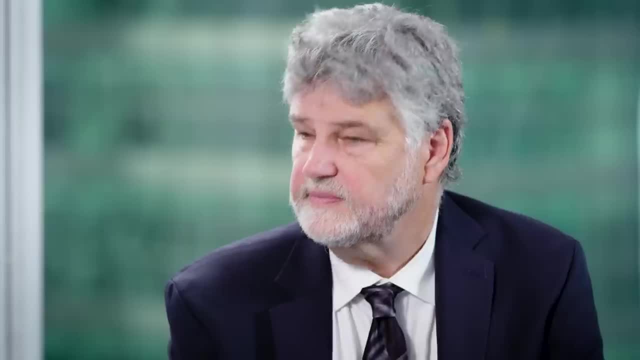 And I've been talking, starting with what is a laser, through linear optics, nonlinear optics, high-intensity laser physics, and saying that we're trying to get to that swinger limit of 10 to the 29 watts per second. We're at about somewhere just shy of 10 to the 23,. I think at this point 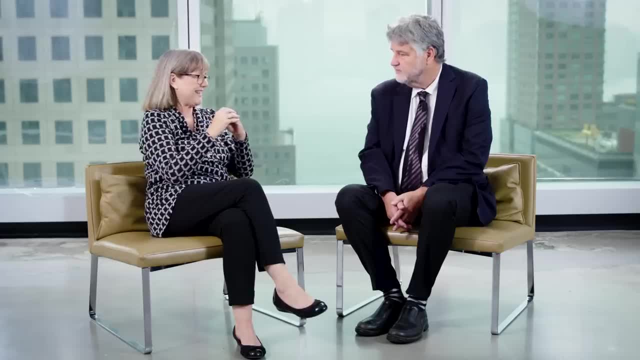 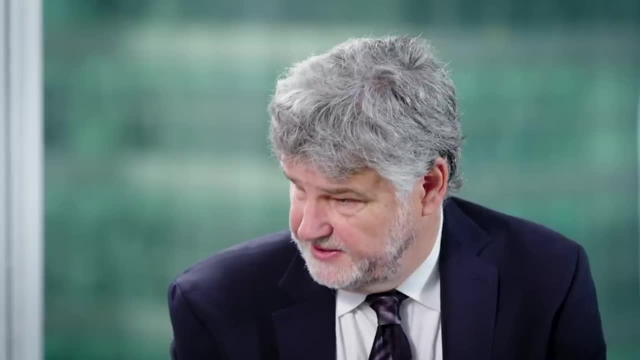 But even if we get to 100 petawatts and focus that down to a wavelength, we're not at 10 to the 29.. Yes, So you're hoping to build the biggest laser at Rochester, but we're still not going to get to the swinger limit. 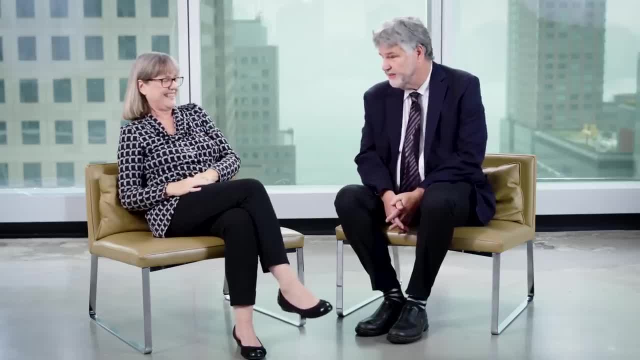 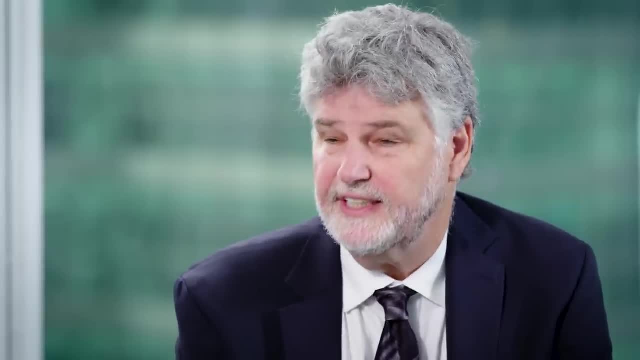 Isn't that right? So just a little bit of back history again. After you demonstrated CPA, I was intrigued by how powerful could we make lasers? and then how lasers are wonderful. Well, lasers are wonderful because they allow you to take energy and compress it in space. 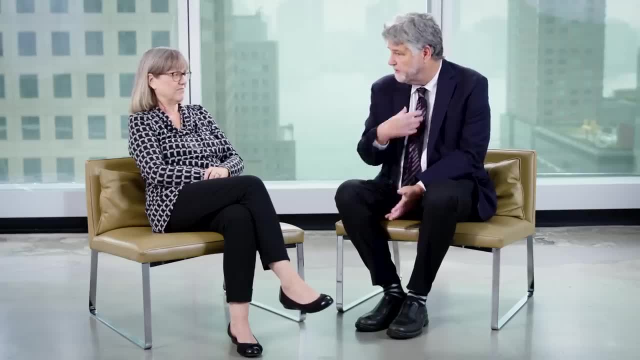 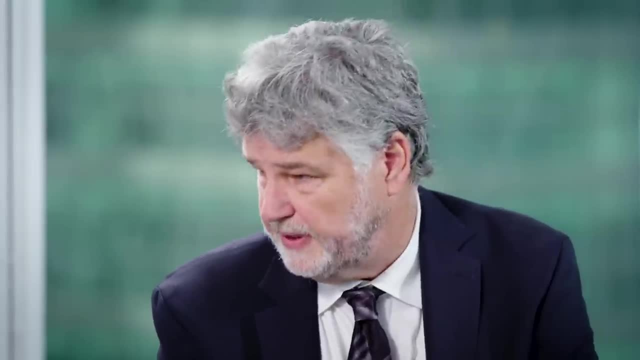 and time. So having high peak power is something that's been a motivator for me for a long time, And so we at the university are making proposals to build two 25-petawatt lasers, maybe 30 petawatt lasers. 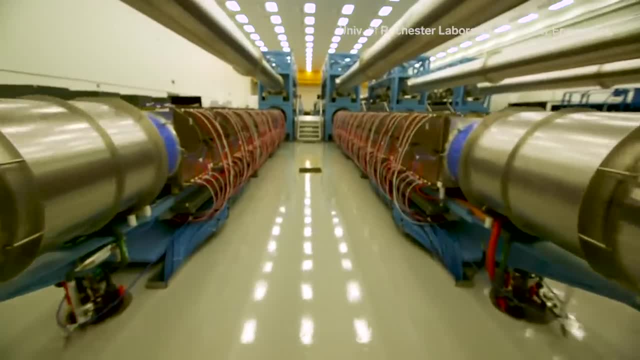 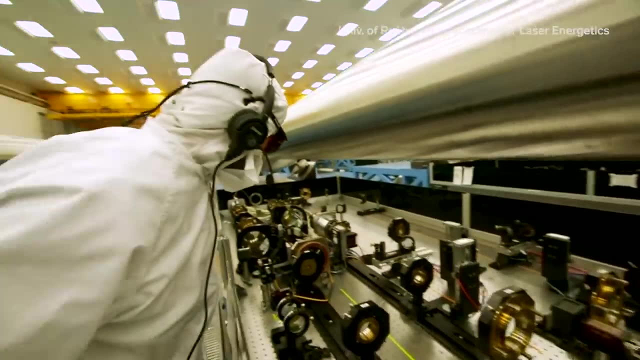 We'll use them to be able to get combined power of over 10 to the 24 watts per square centimeter- still far from the swinger limit. But we have a trick: We're going to use one of these petawatt lasers to make an electron beam. 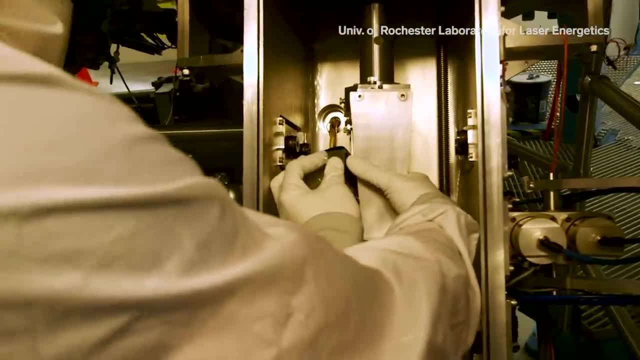 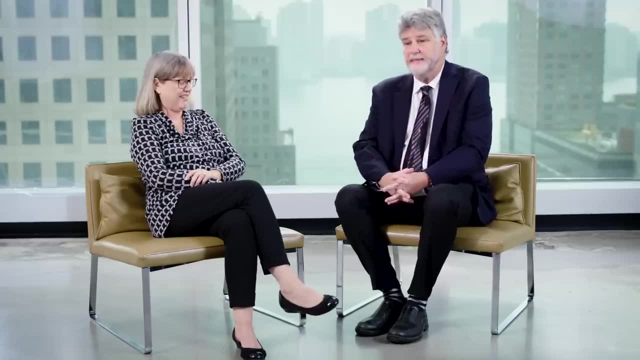 And this electron beam will be relativistic. We actually think we could make an electron beam maybe even hundreds of GeV, up to TeV, which would be another Nobel Prize if we did that. That's right. If you can do that, go for it. 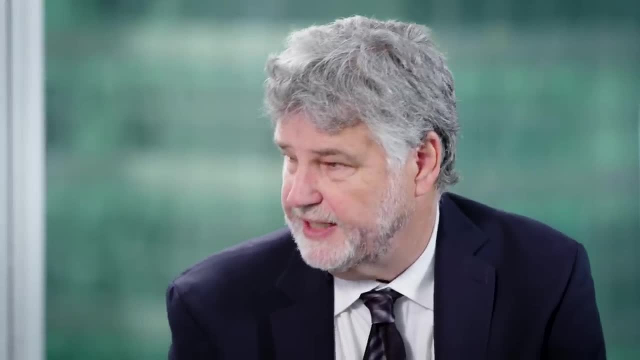 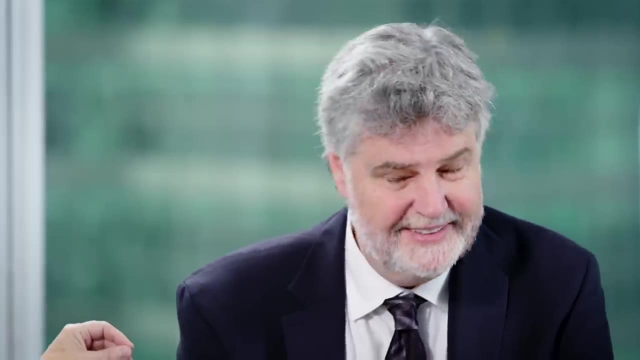 And then we will shine that laser onto that electron beam And the electron's rest frame. we meet the swinger limit. Okay, But that's kind of cheating. That's not getting to 10 to the 29. If you could do it with 100% efficiency, that's all we need. 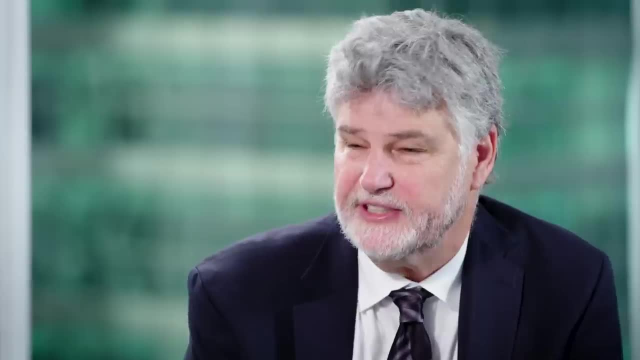 That's why I want to cheat. That's the Nobel Prize-winning idea, though, if we could come up with it. That's why I want to cheat, Because, again, if we're able to do this, you know, with ways I can see today, right. 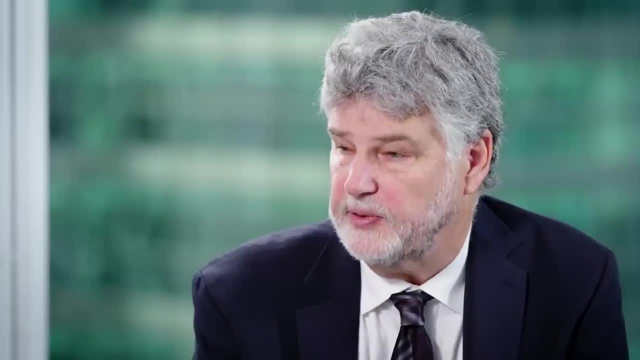 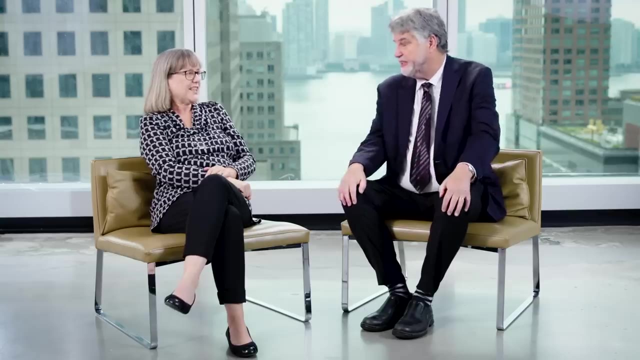 I can see us doing it today, by just exploiting what we already know and taking it to a limit. then that would be a real motivator, I think, to be able to even take these techniques further. Cheating is not the right exact word. 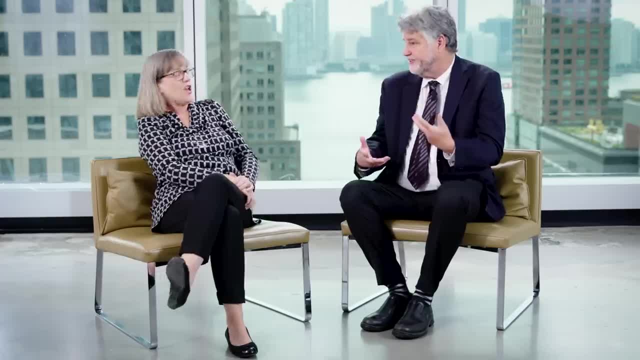 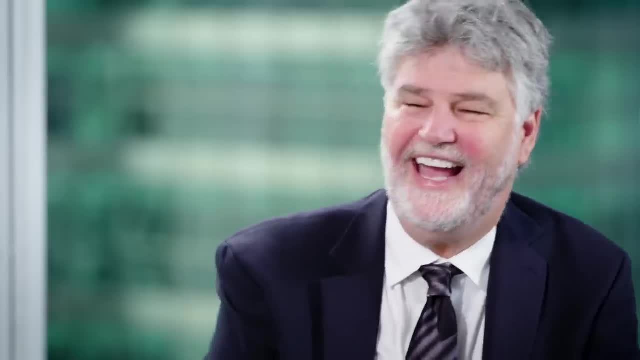 It's taking advantage of relativity. It's taking advantage of all physics, not just optical physics, And so that's why we want to do it this way. We have to get into entertainment. When is the high-intensity laser going to get into entertainment? so then there's real money. 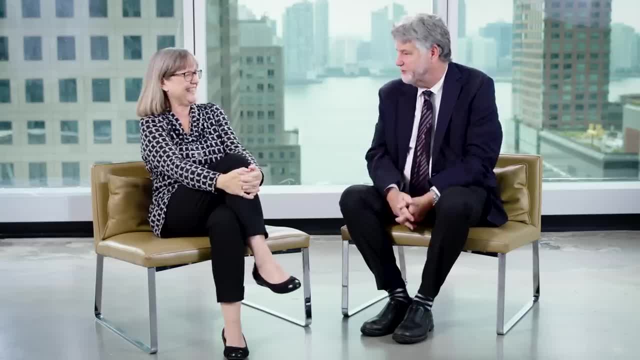 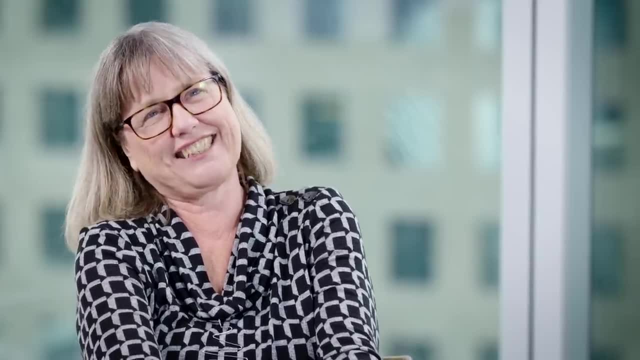 Yes, yes, Well, we have Star Trek, We have the photon torpedo. I always thought they actually knew what you were doing. There's a photon torpedo, right, Remember? Have you ever seen that on Star Trek? No, I don't like science fiction. 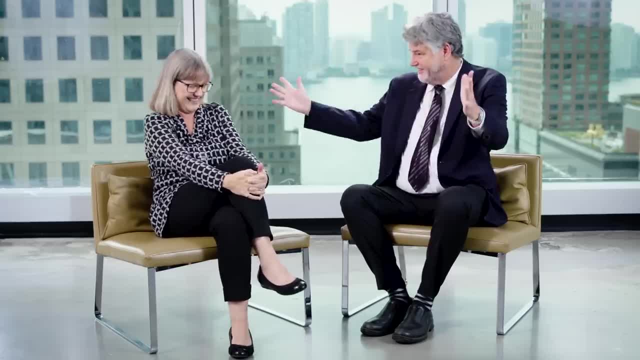 Oh no, Star Trek had photon torpedoes and they showed bursts of light about this long. Okay, It was a CPA, It was a few-thousand-second pulse. Okay, It didn't say how much energy it carried and you could see it. 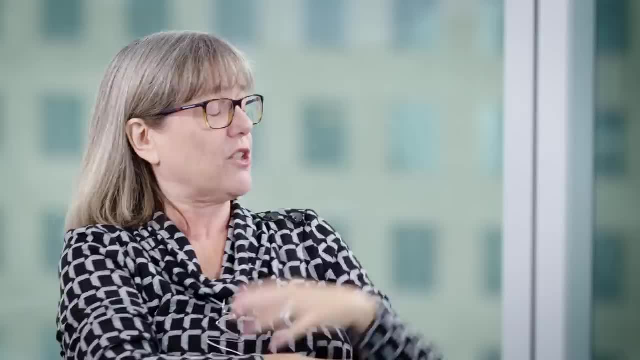 I don't know what it was scattering off of, but you could see it, So it was a great thing. So we could either cheat by doing laser accelerating and going into that rest frame. Yes, And that's like you said. we're stuck a little bit. 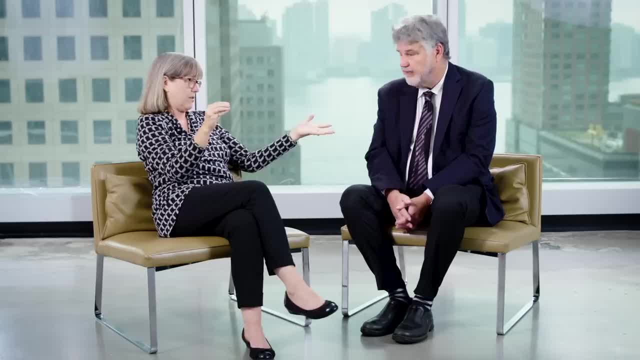 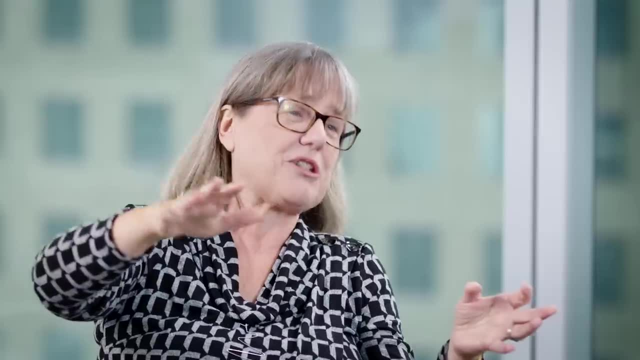 We're not up to that kind of acceleration, So that would be a Nobel Prize-winning possibility. Absolutely, Or we need going around and giving my talks now. I show how we're plateauing. I showed how there was a plateau. CPA raises it up. 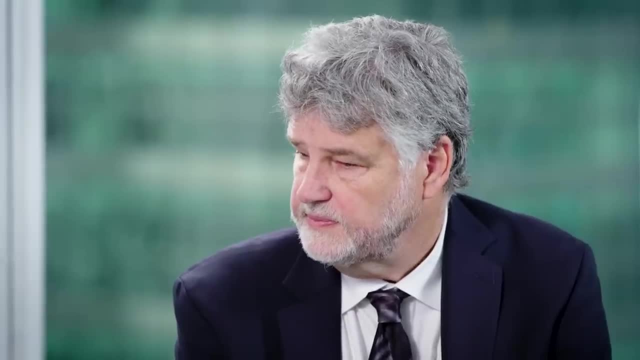 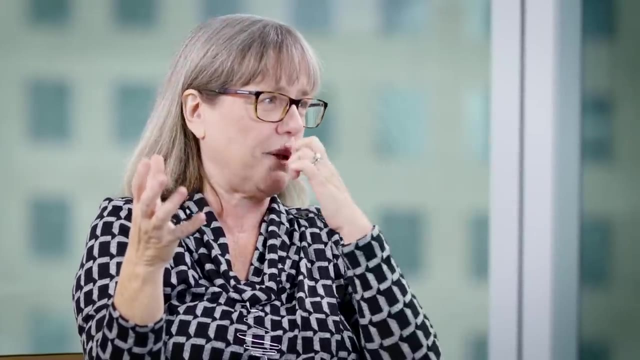 But we're sort of starting to plateau again and we need another Nobel Prize-winning idea, And so do you think it's on the horizon? Do you see anything out there that really says, oh yeah, that's a good way to go? 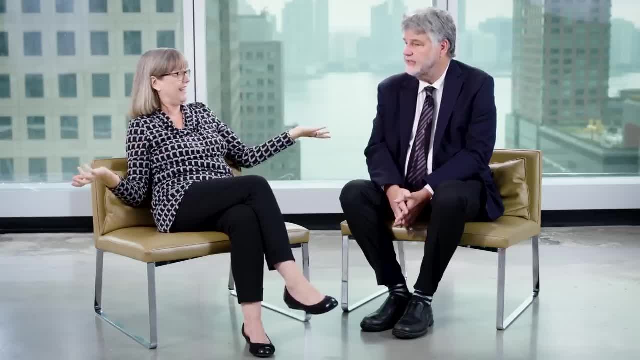 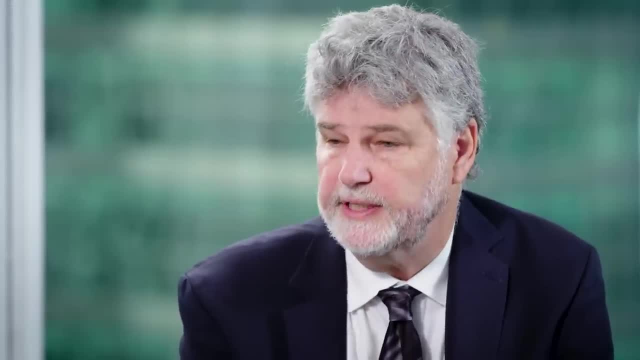 Because we're going to have to get out to the X phase, right, We can't stay in the visual. So actually I think there are potential ways of doing it with optical or near-optical radiation, Right, And you know there's been a lot of work done in the Defense Department and other sources. 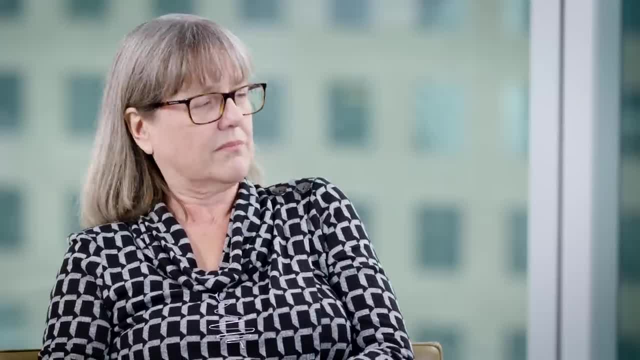 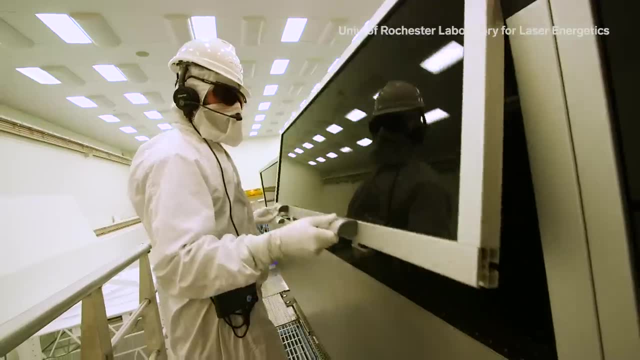 of how do I combine laser beams together and make them act as one coherent source. So one of the things that we'll be doing with our two petawatts: we're going to see if we can actually combine them into a 50. If you can do that, you can begin to imagine doing this with many lasers. 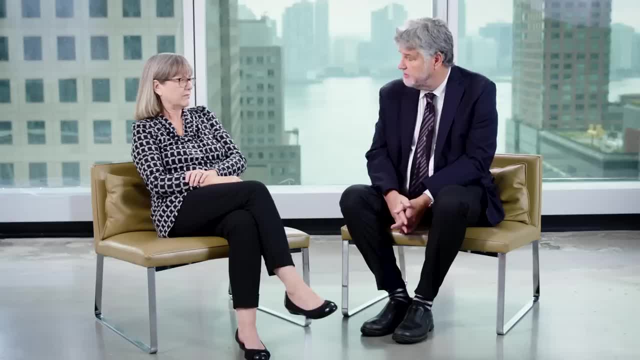 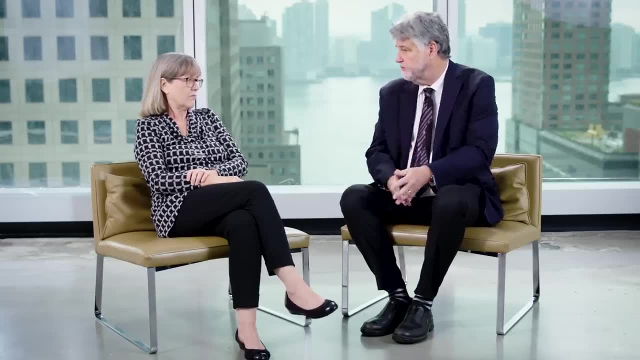 many petawatt lasers of the scale we're talking about, So one could possibly see an exawatt from that. You know, people have been able to combine tens of lasers together for a coherent source, So you have to be able to phase lock them. 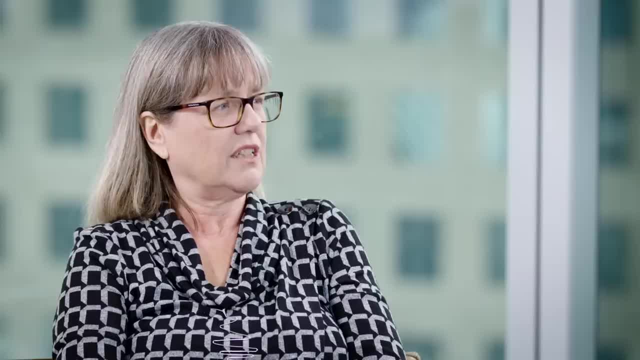 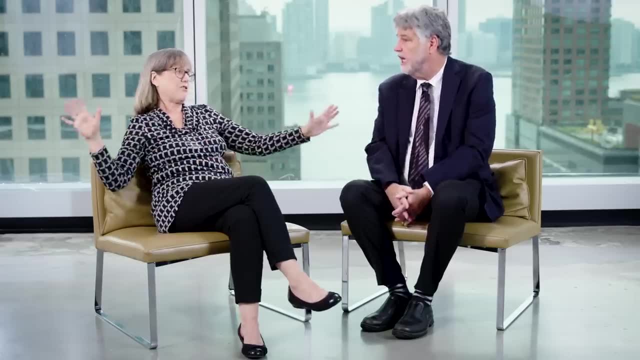 You have to be able to make them, you know their phases, be exactly connected and related and be able, as they propagate through all the different optical components, whatever it may be, to stay locked together And right across the beam. Don't you think that's going to be the challenge? 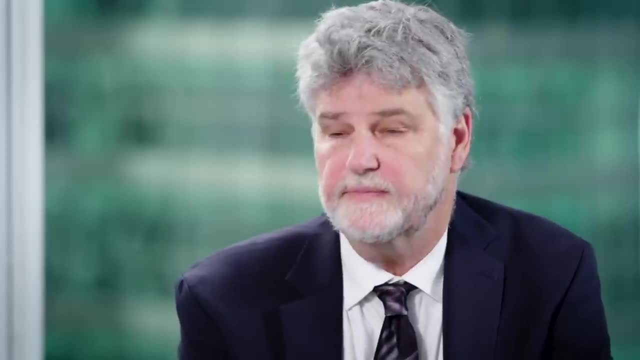 And across the entire aperture, Because it's not like our beams are as perfect as we all like to think they are, So that's right. So you have to have so over the aperture size. you have to have them phase locked across the entire aperture. 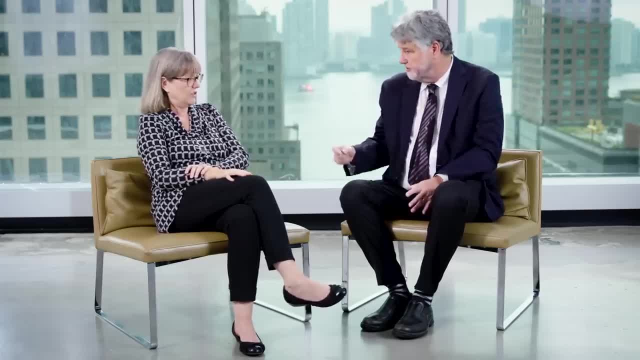 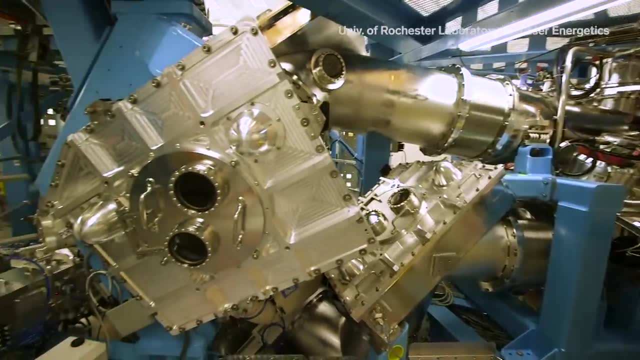 which will be a great challenge, And people have done it again with small lasers. The laser we'll be trying to do is about 40 centimeter aperture, So we'll begin to start looking at this And actually wave fund control. I mean be able to adaptive optics. 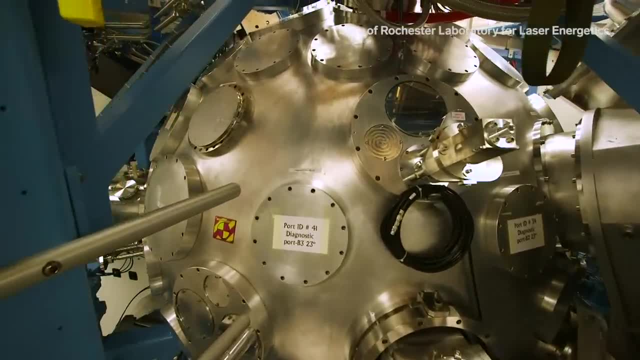 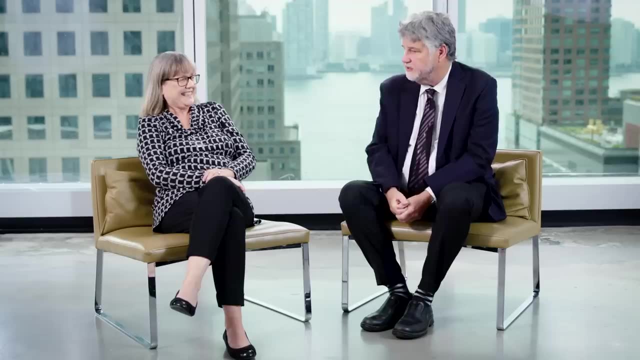 other ways in which you can control the uniformity of the phase is something that's been developed in lots of ways now, for defense applications, for science applications. So we will do our best to make use of all these technologies. Lasers, I think, have progressed so much, just like the semiconductor business. 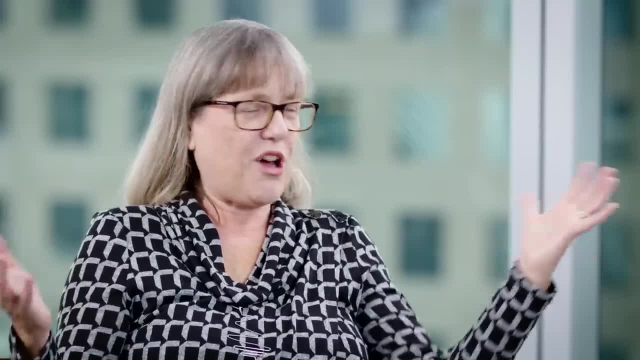 because there's such a market for them. There's so many different applications. Okay, so there's a lot of us working around the world on these high intensity lasers, And so what do you think the real fun is? What do you see the real excitement being? 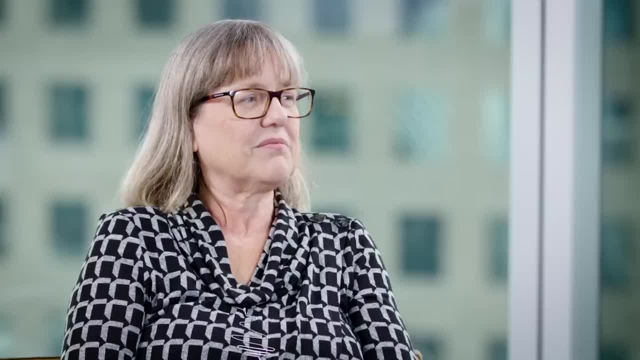 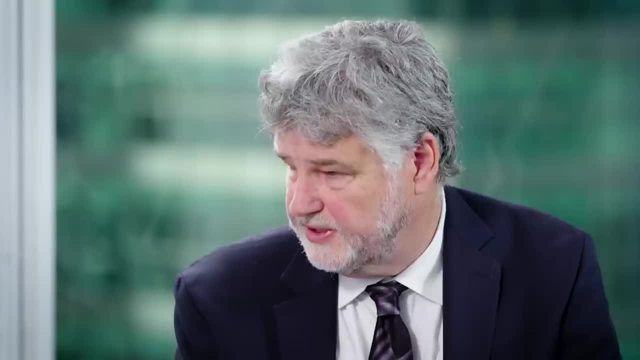 I remember when laser was first demonstrated in 1960. What could we do with this? We already got light. Now we can't live without lasers. My cell phone that is in my pocket has billions of transistors. How is that made? 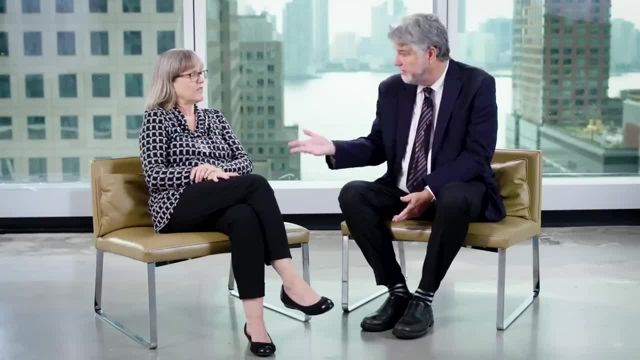 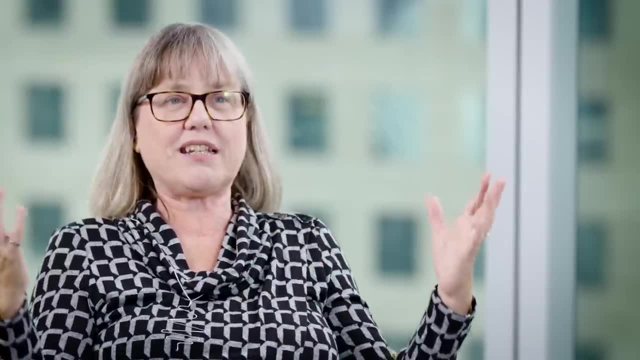 With lasers. All integrated circuitry is done with lasers. Actually, now it's being using x-rays made from laser heated matter that came out of the laser fusion program. So it is amazing. the parallels and optics is used everywhere. We're going to possibly take over from CERN. 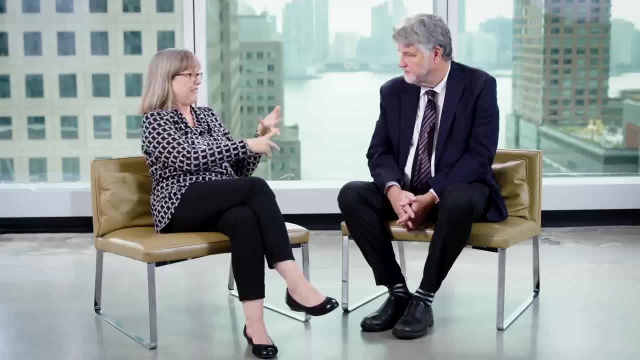 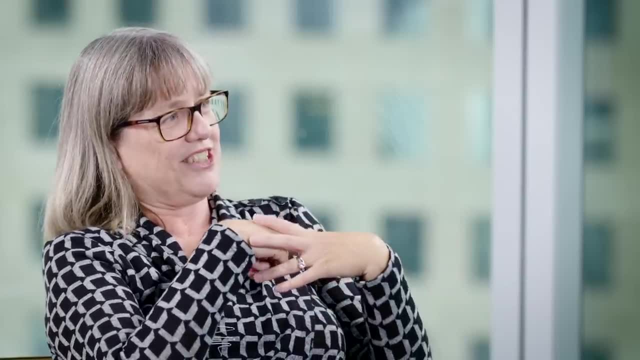 and we'll just do high energy physics with lasers. Yep, We're looking at gravity waves with lasers. We want to do black holes with lasers. We want a machine with lasers. We want to do medicine with lasers. It's everywhere, And now, with the Nobel Prize, people are hearing more about it. 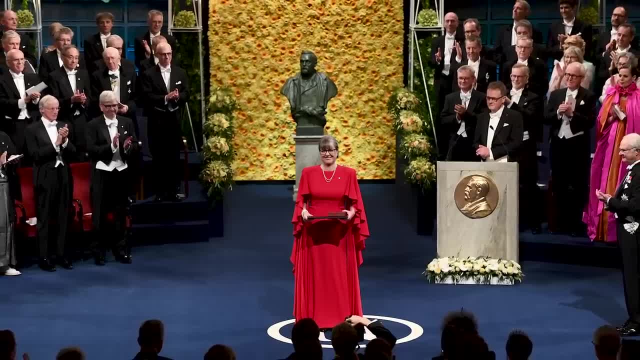 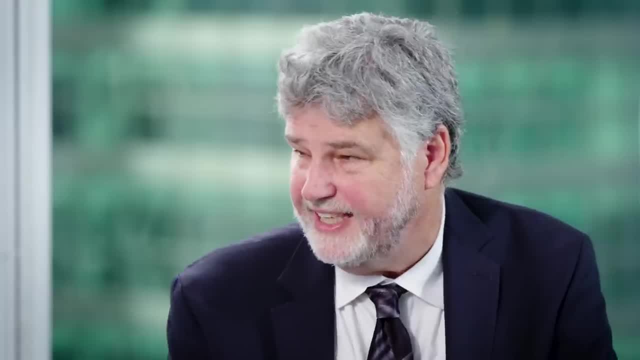 so now lasers are everywhere. I couldn't agree with you more, And you winning the Nobel Prize has been an inspiration to lots of people. Only three women have won the Nobel Prize in physics, and only one educated in the United States. You.